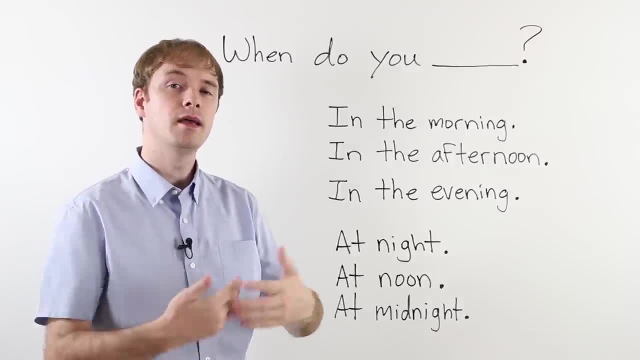 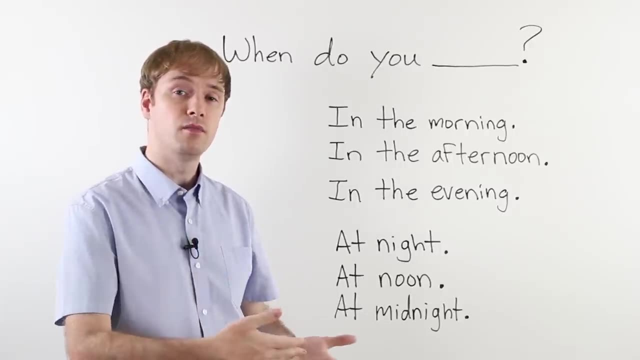 Don't say in morning, In the morning, When do you wake up In the morning? When do you take a shower In the morning? When do you go to work In the morning? Okay, Let's look at the next one. 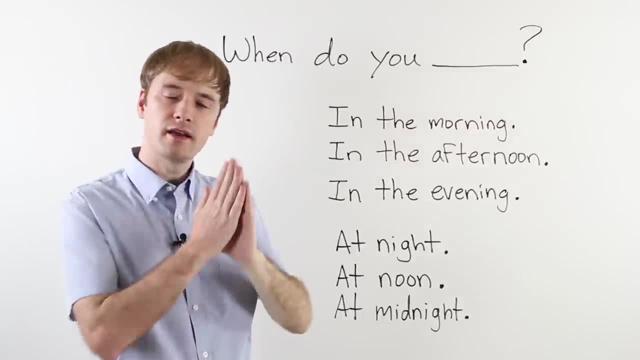 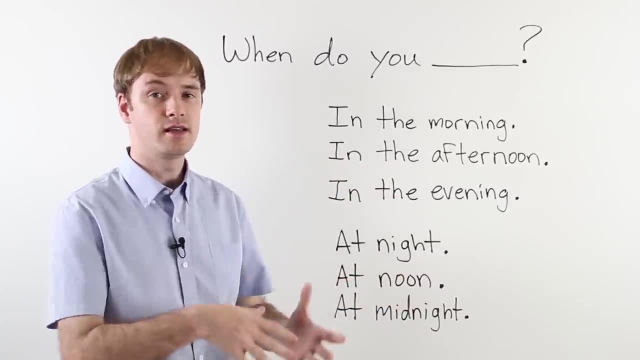 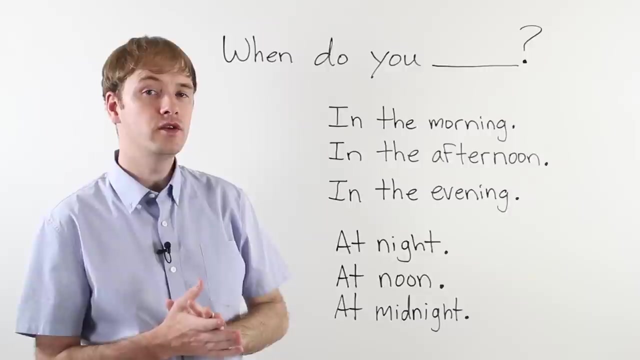 In the afternoon? In the afternoon, when do you take a nap? Okay, You take a quick sleep. When do you take a nap In the afternoon? Okay, I like to take a nap In the afternoon. When do you go home after work? When do you go home In the evening? When do you eat dinner? In the 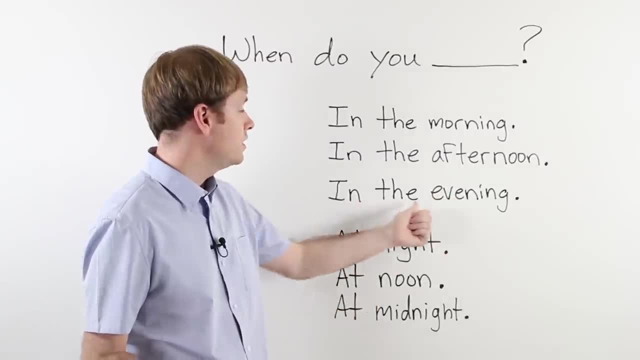 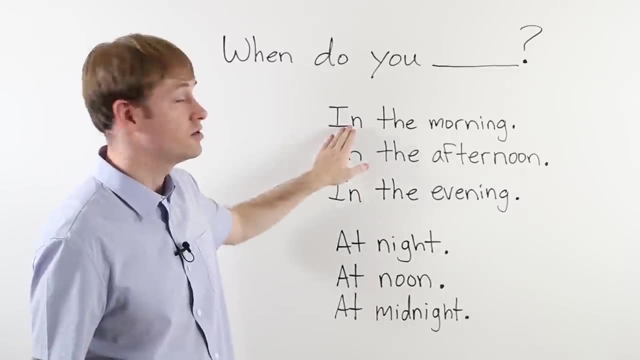 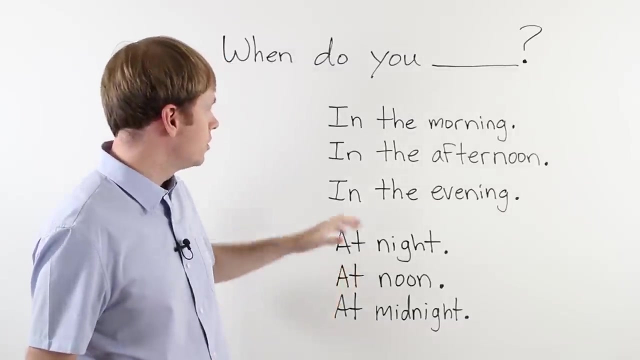 evening. When do you watch TV In the evening? Okay, So these are very easy ways to express the different types, the different times of day. Make sure you have in the Alright. Let's look at the next ones They're using at. Okay, So this first one is using. 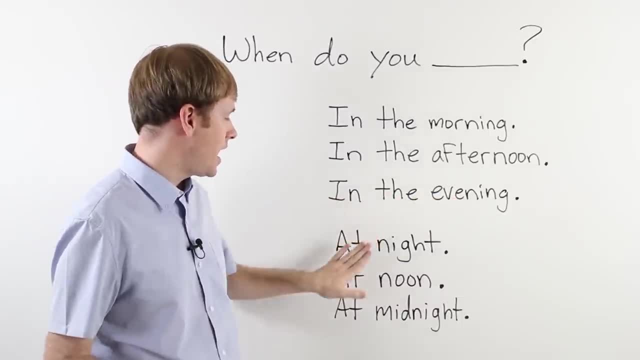 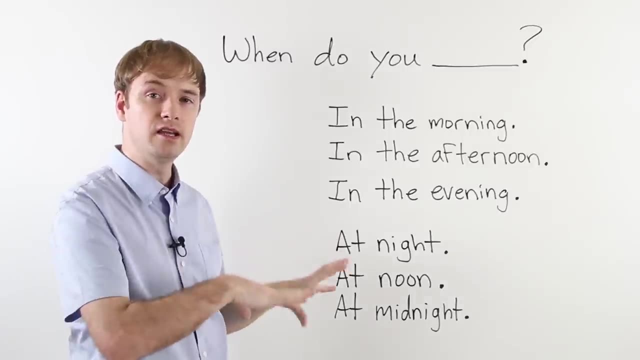 at night, In the evening. at night, Very similar, But in the evening is usually talking about early evening, Okay, Around 6 pm to 10 pm. Okay, That's the evening time. So in the evening, relaxing time At night is probably after 10 pm. You know you're going into 1 am, 2 am, 3 am- Very late time. Okay, That's usually when we say at night. 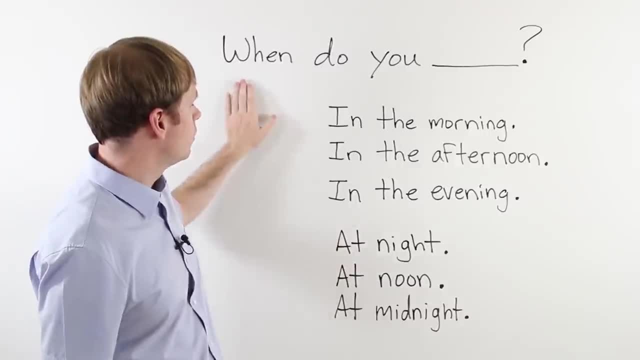 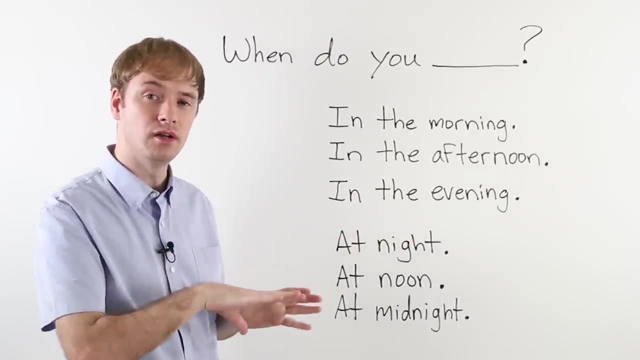 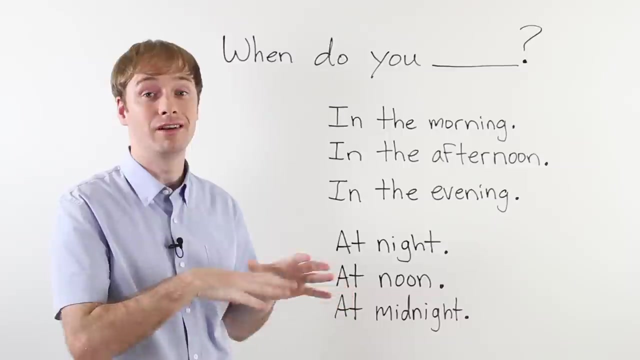 Alright, So when do you? well, if I said when do you go home from work and you said in the evening, okay, and I know it's early. If I asked when do you go home from work? that at night, I would think, oh, very late, maybe after 10 PM. Alright, you have to be. 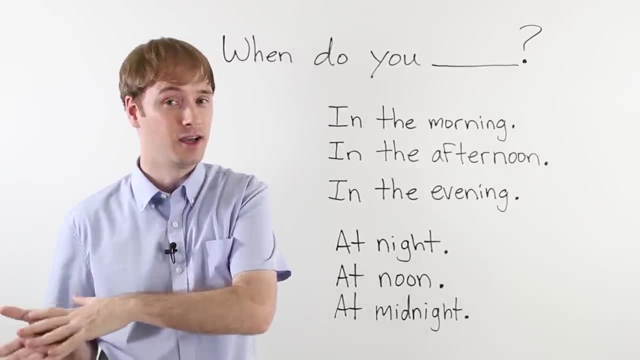 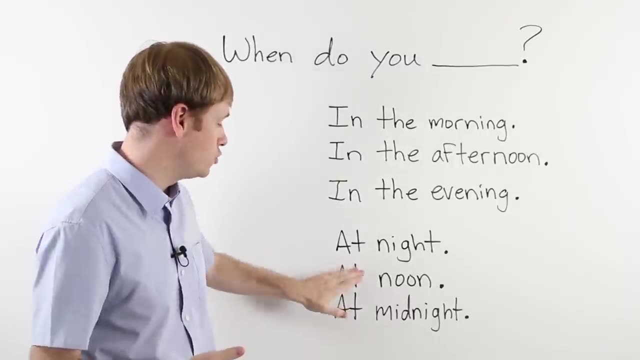 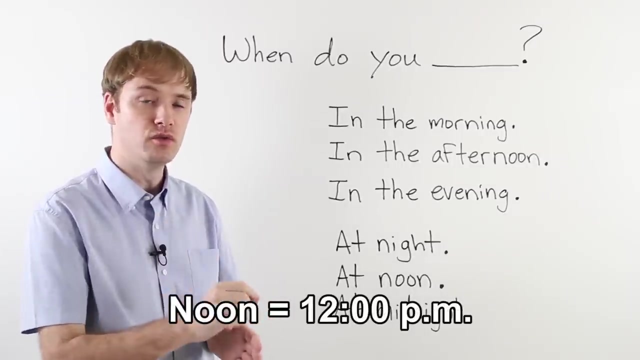 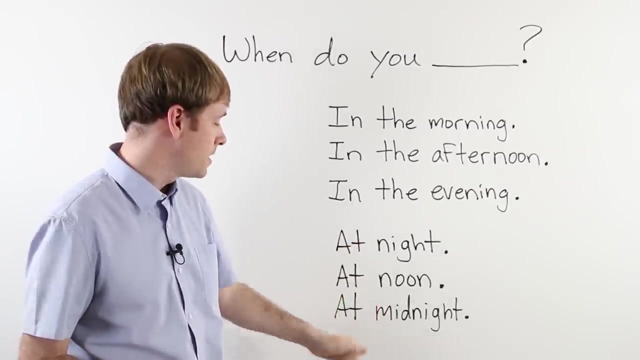 very careful walking on the street at night. Alright, the next two are very exact times. Ok, at noon. at midnight Noon is only 12 PM. That is noon. So when do you have lunch? You can say at noon, Alright, Midnight is. 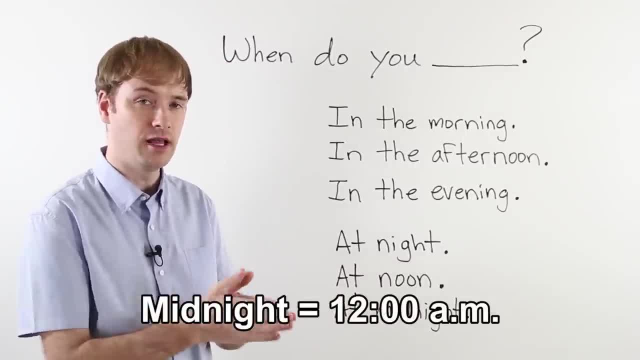 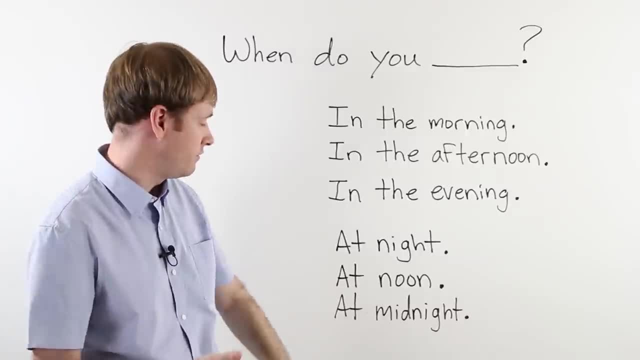 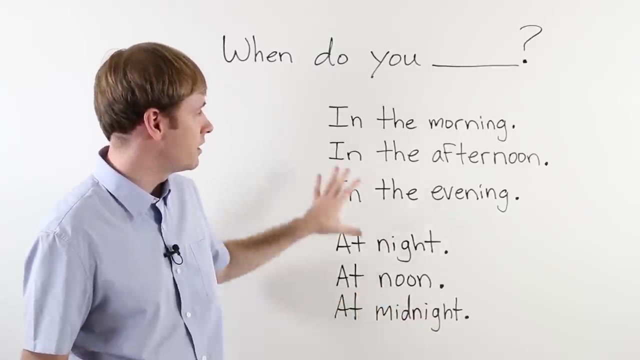 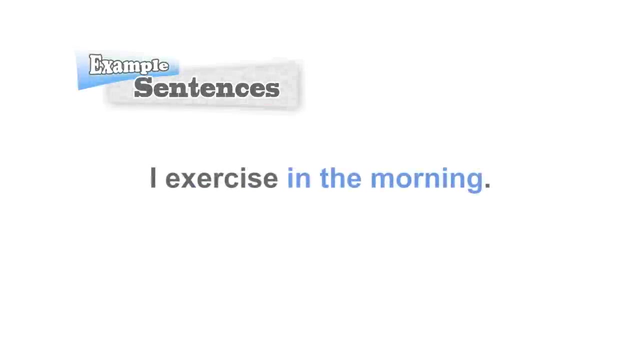 only 12 AM? Ok, very late. When do you go to bed? At midnight? Ok, very, very late. Only 12 PM, only 12 AM. They're very exact times, Alright, so these are different ways to express the times of day. Let's take a look at a few examples. Okay, let's. 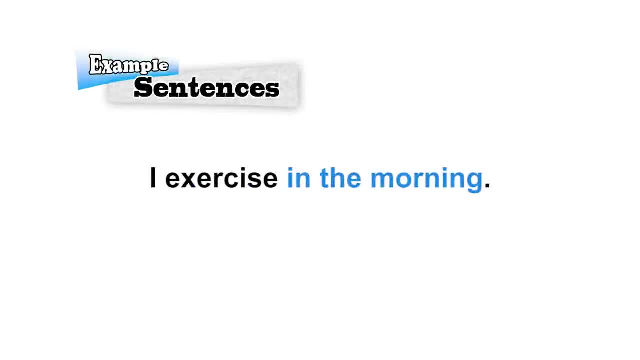 look at these examples. The first one: I exercise in the morning. I exercise in the morning. The next one: My lunchtime is at noon. My lunchtime is at noon. The next one: I like to go swimming in the afternoon. I like to go swimming in the afternoon. The 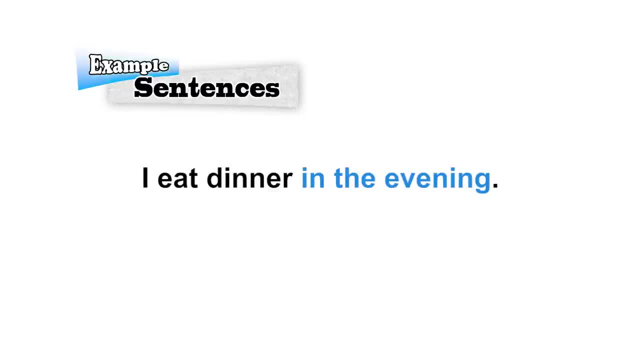 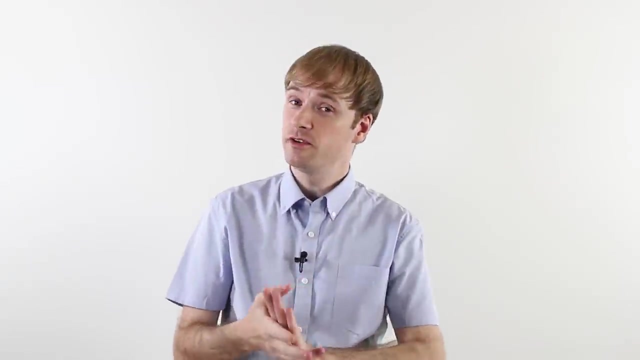 next one: I eat dinner in the evening. I eat dinner in the evening. And the next one: I eat lamyon at midnight. I eat lamyon at midnight. And the last example: be careful walking alone at night. Be careful walking alone at night. Okay, I hope you understand. 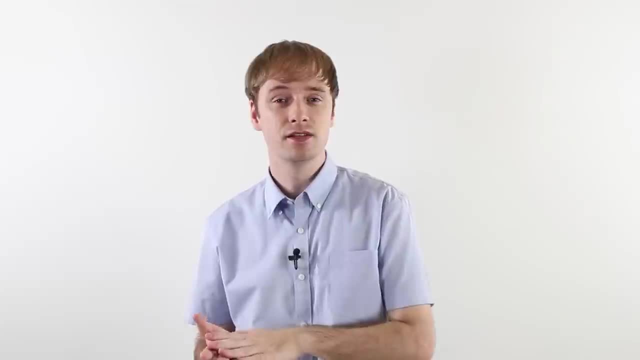 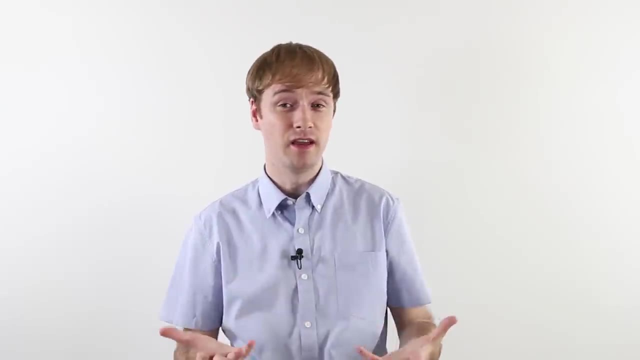 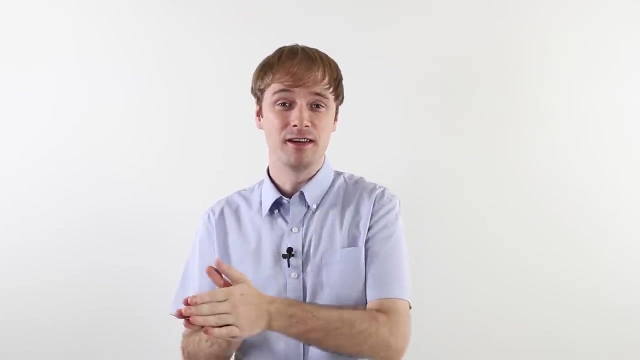 how to express the different times of day in English. I'm going to ask you a question now: When do you study English? Okay, what time of day do you study English? When do you study English? I suggest the best time to study English is in the morning. Okay, in the afternoon. 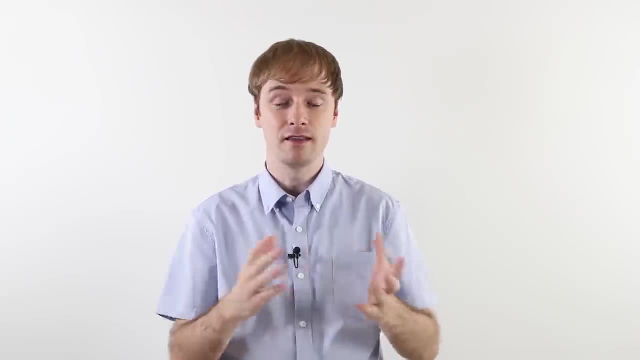 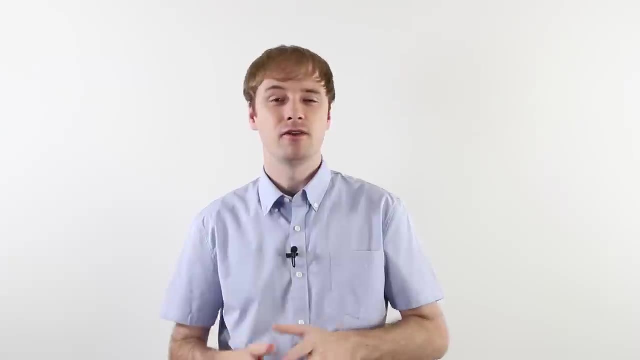 is not so good. A lot of my students are always very tired in the afternoon. In the evening is okay, but never. never at night, That's too late, Alright. so I hope you understand these time expressions. See you next video. 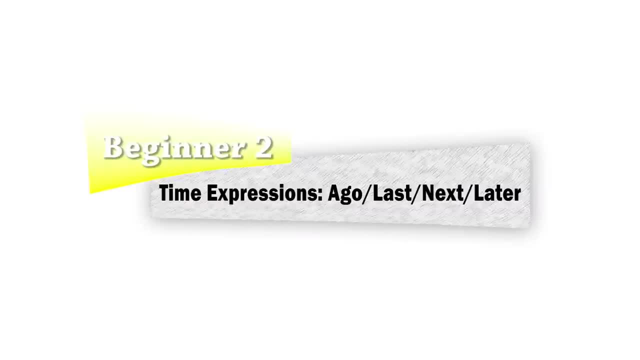 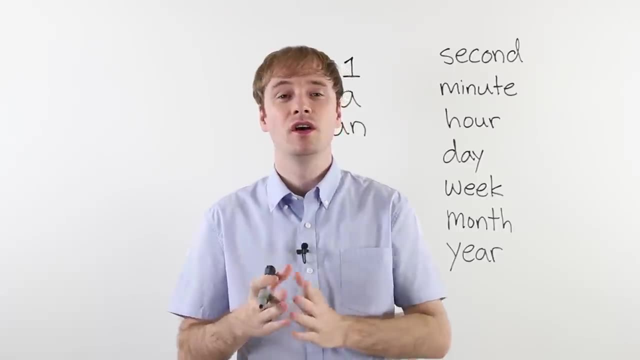 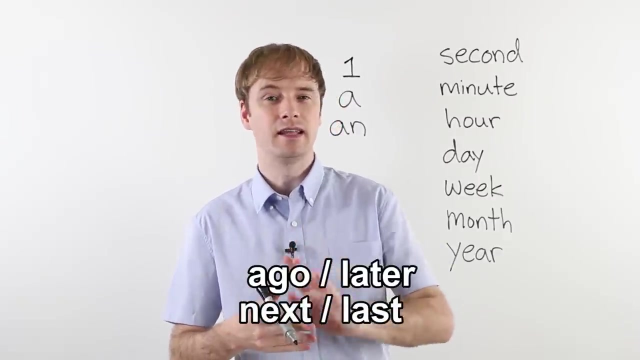 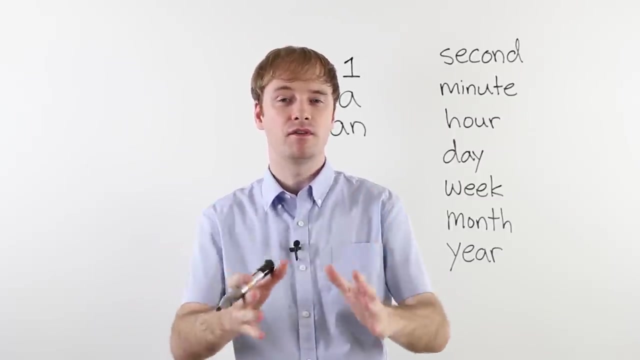 Hello everyone, Welcome to this time expressions video. In this video, we're going to talk about how to use ago, later, next and last. Okay, these are very useful expressions to use when talking about time, But first let's review our vocabulary, And this is the vocabulary. 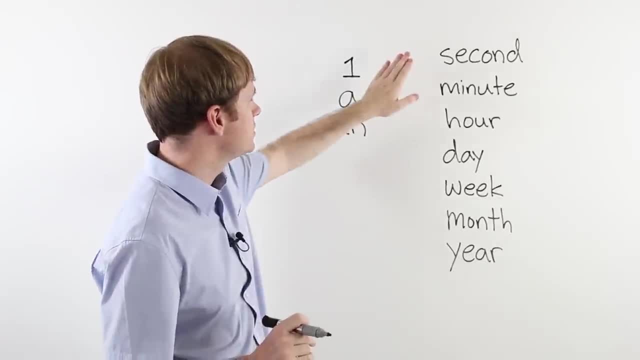 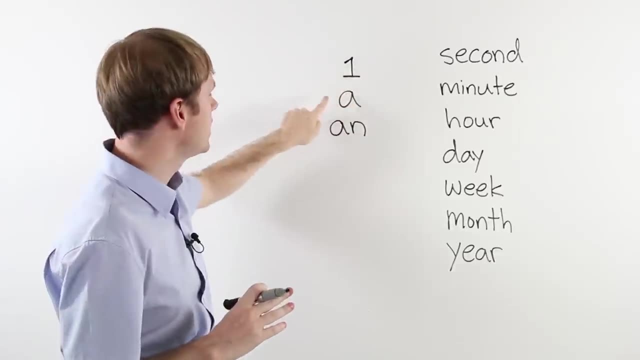 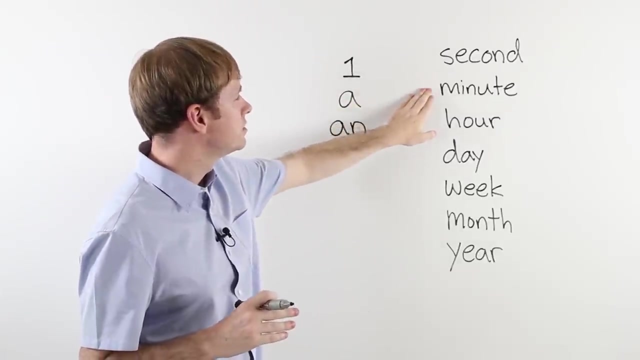 you need to know for this video. Second, and I have one second. Ok, one second. we could also, instead of one second, we could say a second. So one and a in the same. just one second, Ok. one minute, a minute? ok, how many seconds in one minute? Well, 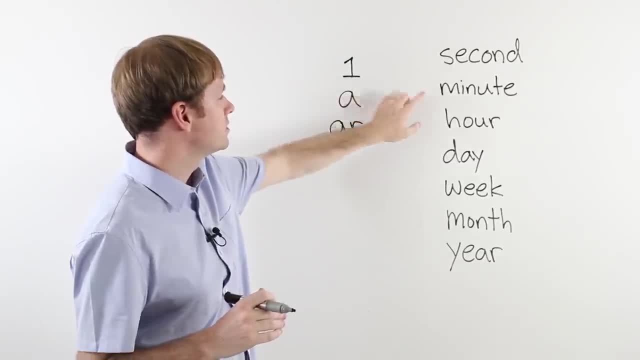 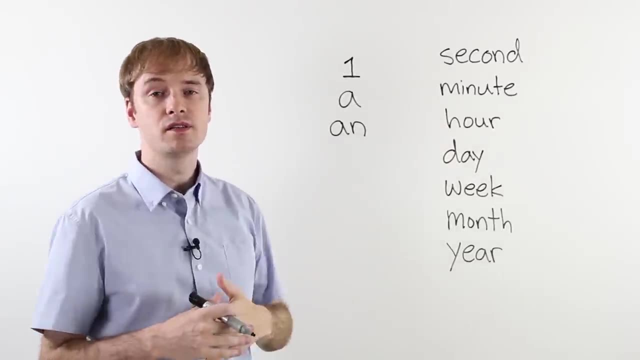 sixty seconds in one minute And the next is hour. Now, an hour is a minute. If you're talking about a minute, then you probably want to. is special because we're going to use on Because hour starts with a vowel. sound On. 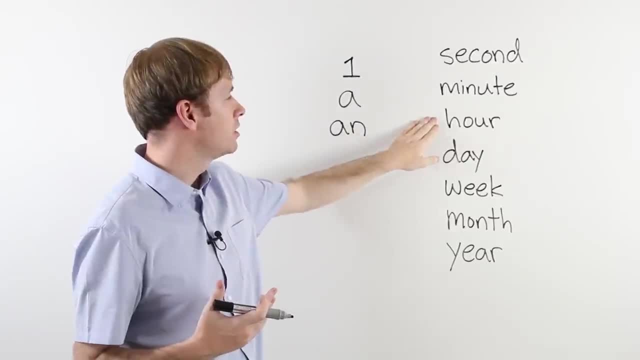 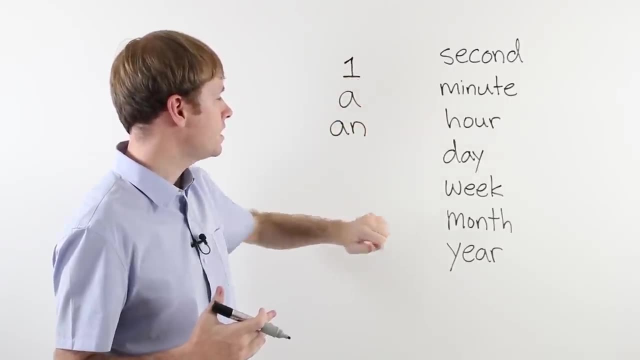 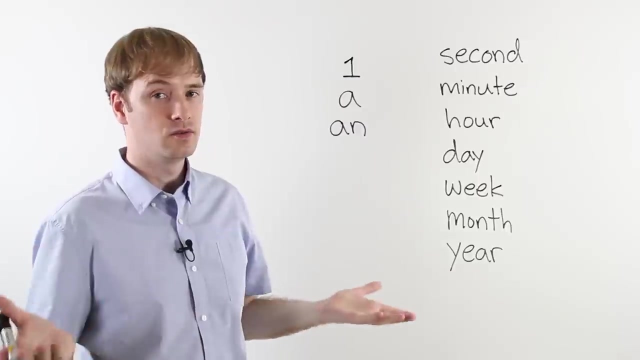 hour. We always use on with hour And of course, there's 60 minutes in one hour On hour. Next is a day, A day, One day, Of course. how many hours in a day, 24 hours A week? How many? 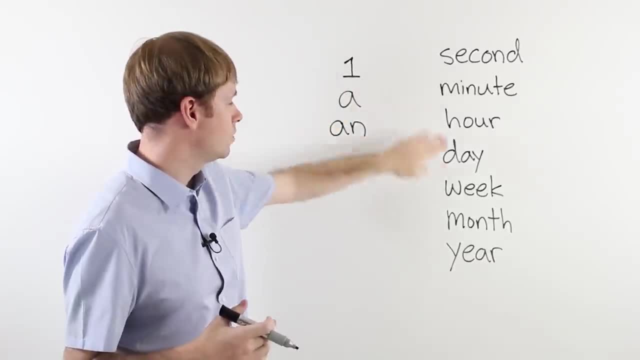 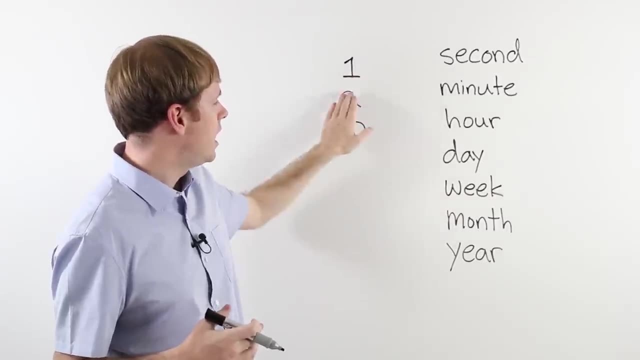 days in a week, 7 days in a week, One week, One month, A month, Ok, And the last one One year A year, Ok. So that's the vocabulary I hope you understand Before we move on. 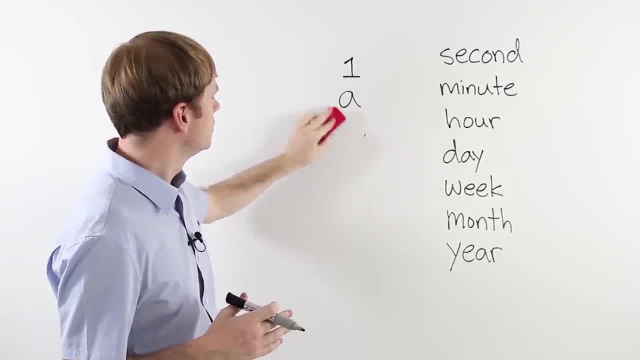 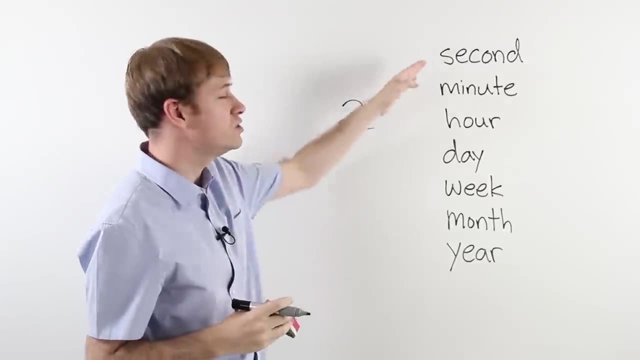 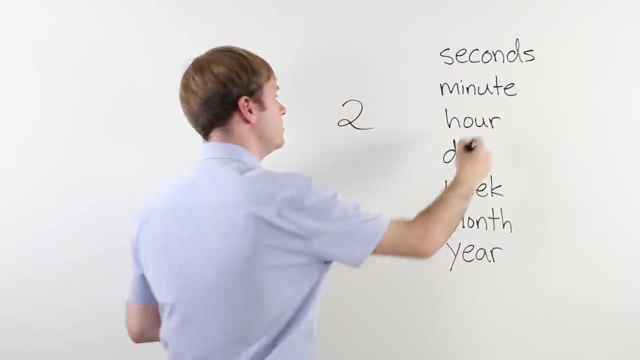 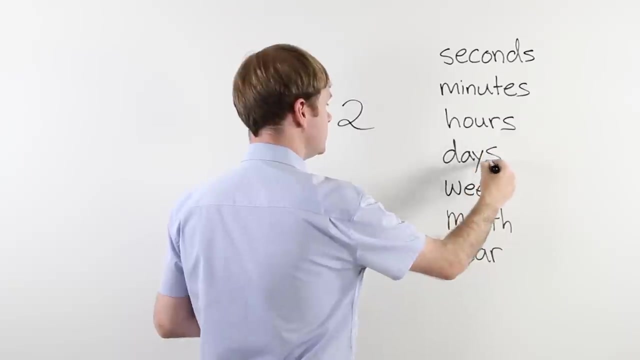 I'm going to change this. Ok, This is one Now, let's put two. Now everything changes. Two second. No, We have to plural Plural it Two seconds. Two minute, Two minutes, Two hour. No Two hours, Two day, Two days. 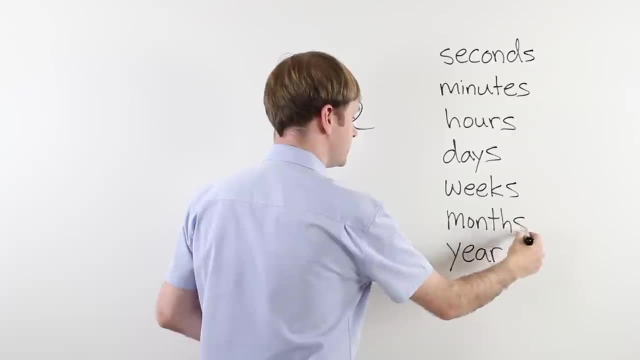 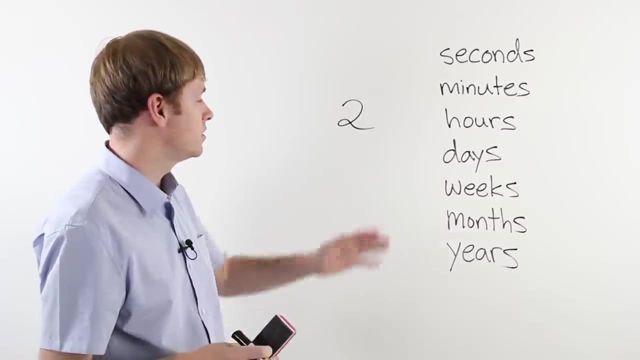 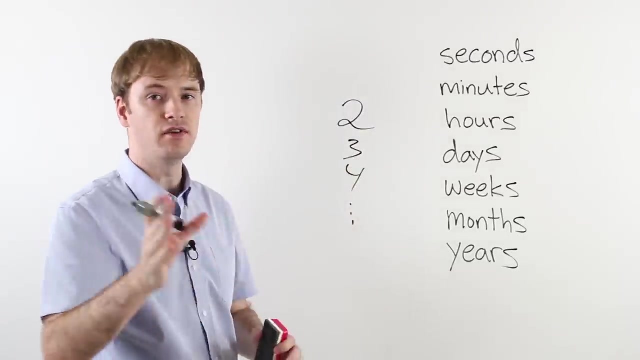 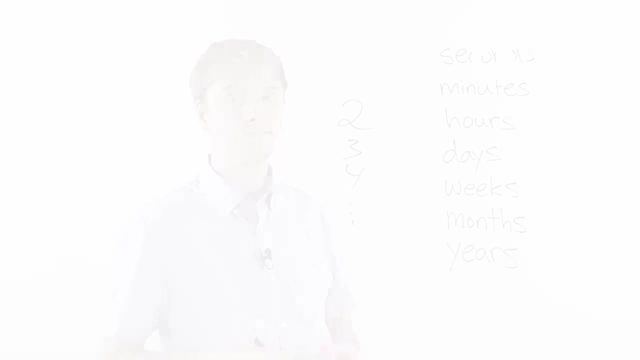 Two week, Two weeks, Two months, Two years, Seconds, Minutes, Hours, Days, Weeks, Months, Years. So if you're using two, three, four, Every number except one, Ok, Make sure you use the plural. Alright, Let's move on. Ok. 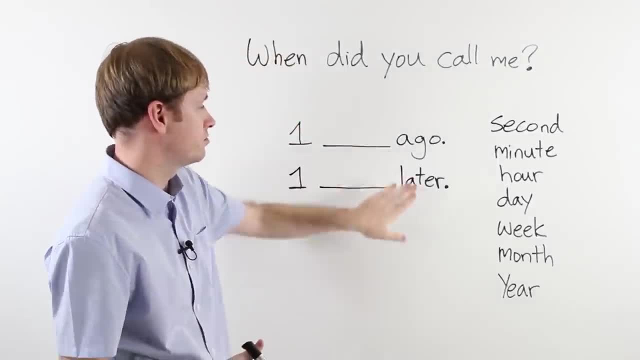 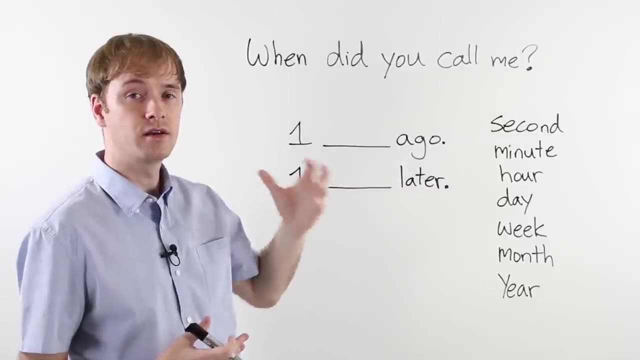 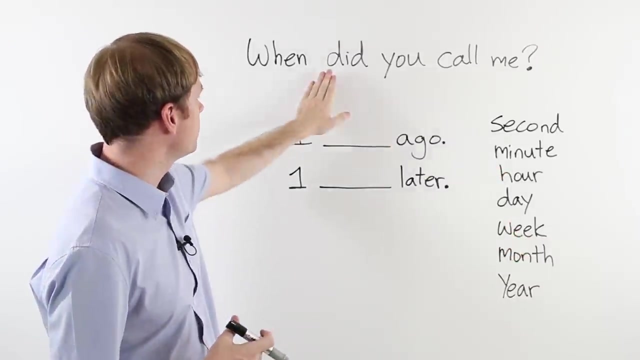 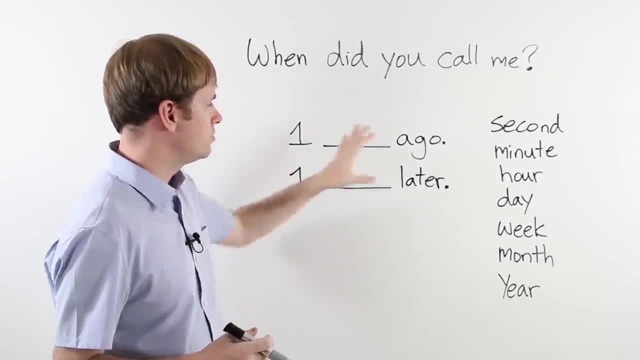 me Ok. When did you call me Ok? When did you call me Ok? When did you call me Ok? When me" Ok, you just put the vocabulary here One second ago. Ok, that's very soon, That's. 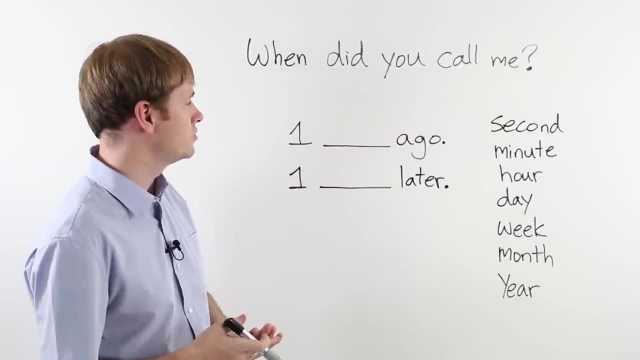 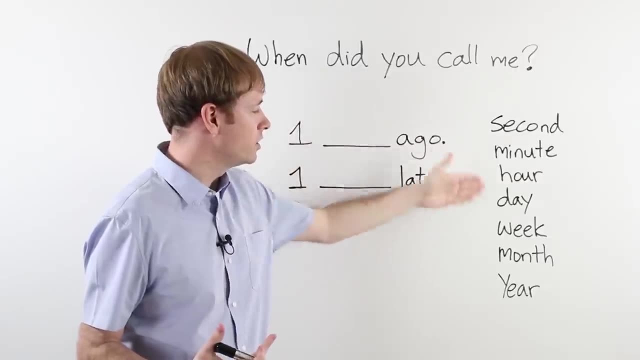 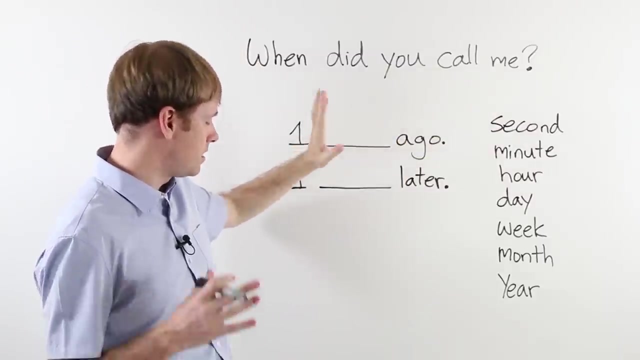 too soon. When did you call me? one second ago? That's too soon. One minute ago, That's possible. One hour ago, One day ago, One week ago, One month ago, One year ago- You can use any of these here, Ok, so remember. if you said five, For example, five, When did? 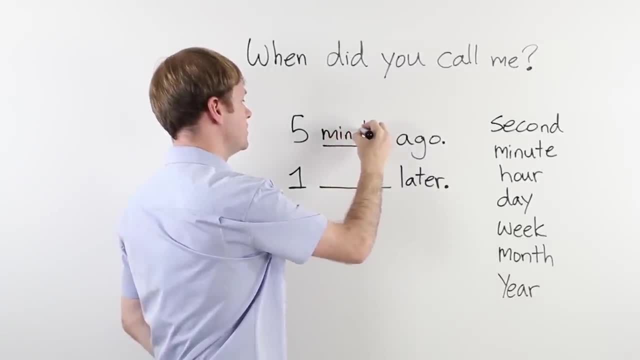 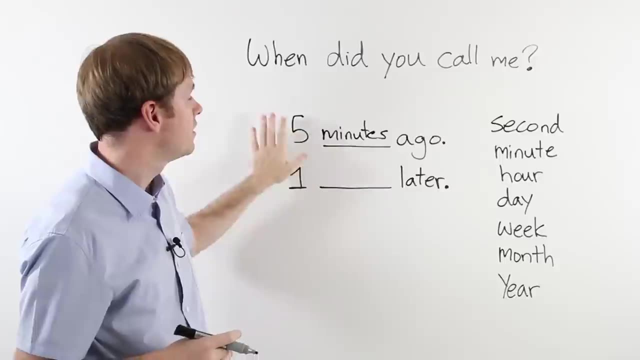 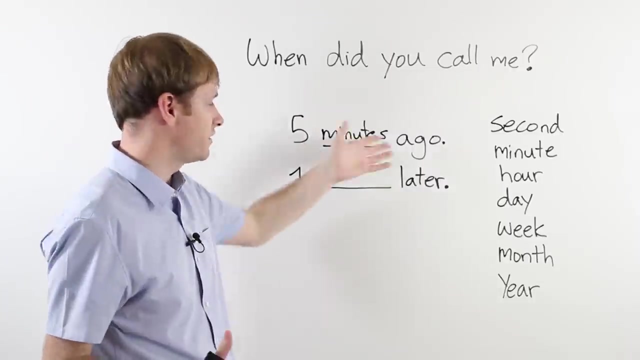 you call me five minutes ago. Five minutes ago, Ok, remember we have this S because it's now five, Five minutes ago. Alright, so we're going to use ago, because it's a past question. When did you call me Five minutes ago? When did you come home? 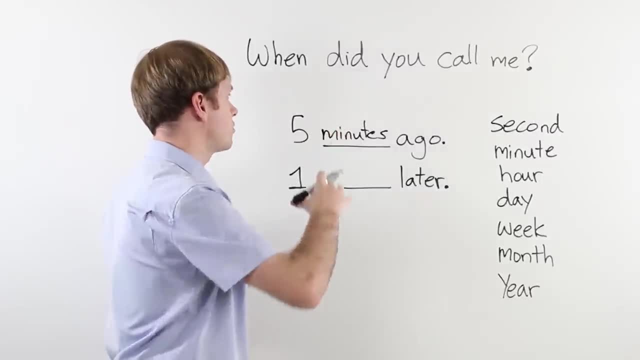 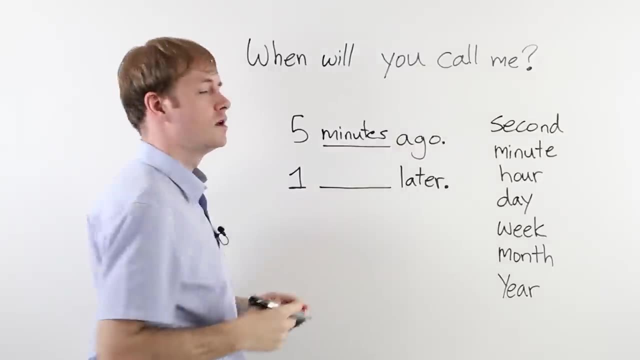 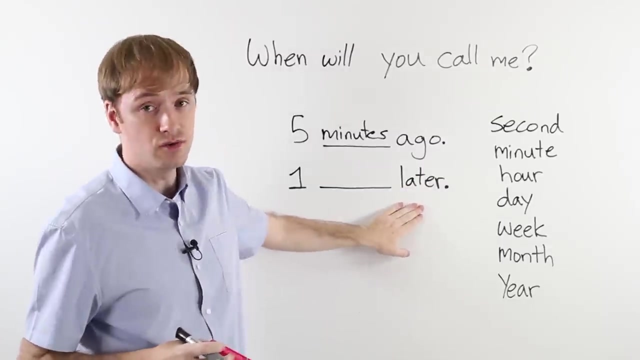 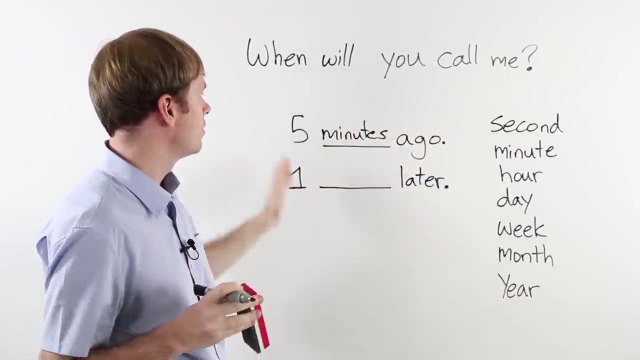 One hour ago. Alright, let's change the question. Let's change it here to the future. When will you call me? Ok, in the future. When will you call me? Let's talk. let's use the future expression. Uh, one second later. Well, that's too soon. Second is a very short time, Ok. 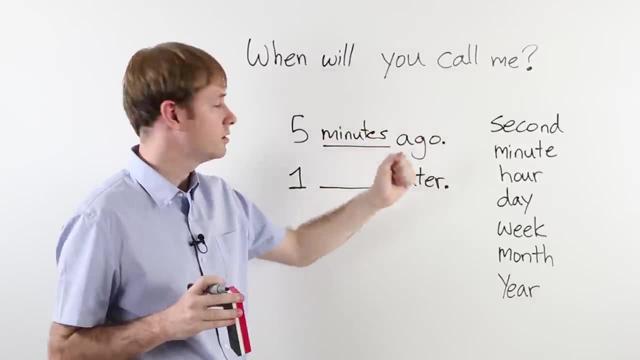 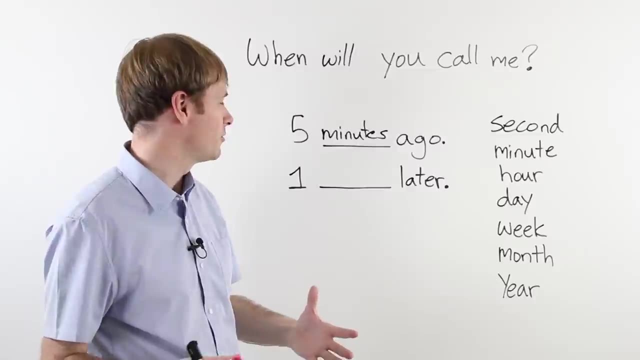 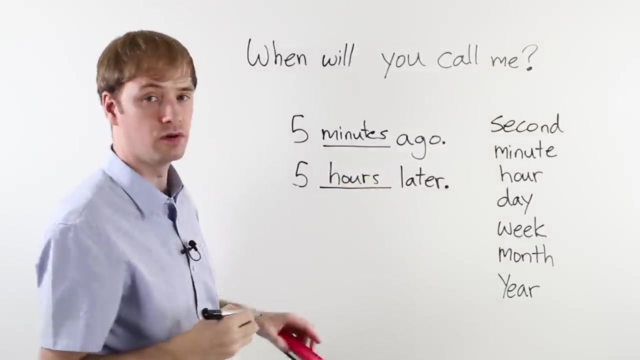 when will you call me? One minute later, One hour later, One day later, One hour later, One week later, One month later, One year later? Very long time, Ok. and also remember, If we're going to use a plural- Five, six, seven, eight- We need the S. When will you? 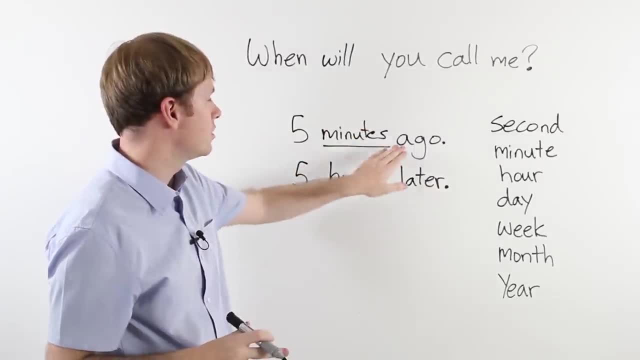 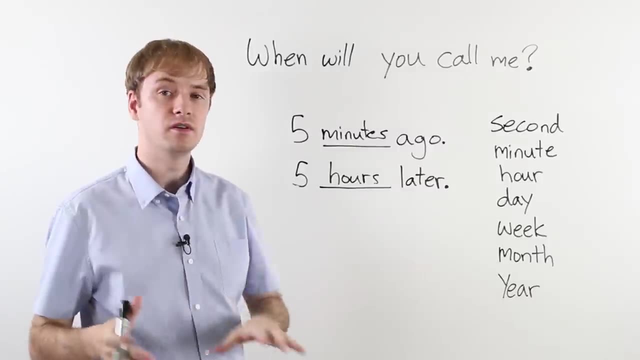 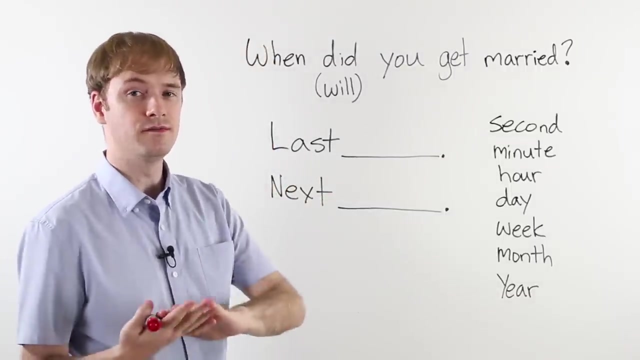 call me Five hours later. Alright, so ago and later- Very useful expressions to use for talking about the past and the future. Let's move on to the next two expressions. Ok, so we're going to look at these two Last and next, Also very useful time expressions. Now 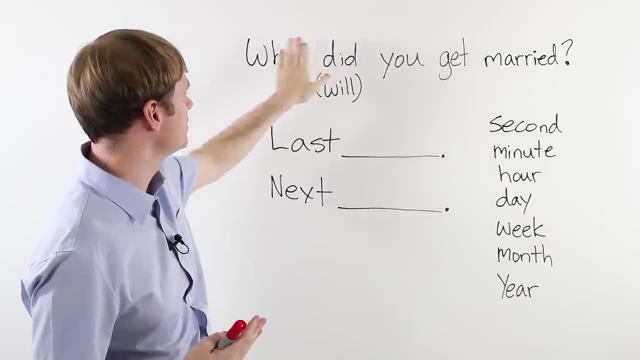 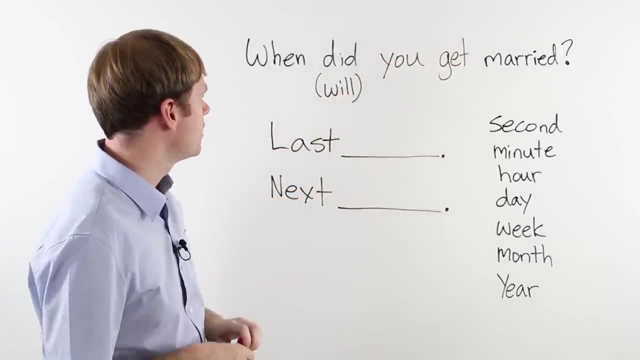 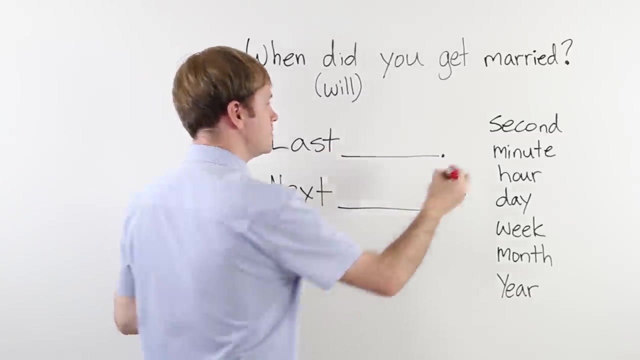 I changed the question a little bit. Ok, so past tense: When did you get married? And for the future: When will you get married? Let's take a look. When did you get married? Last second: No, Ok, we can't use second with this expression. Next second: No Ok. 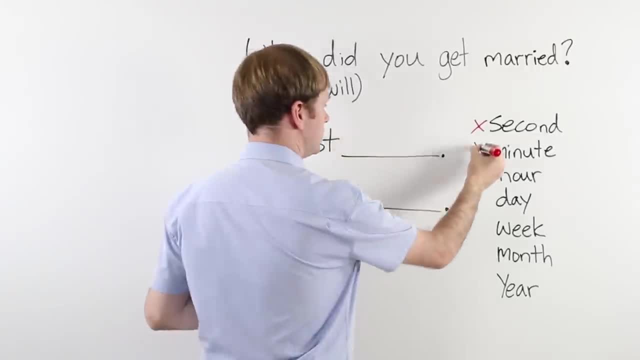 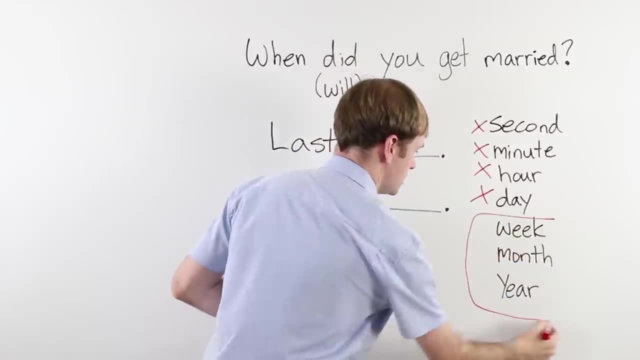 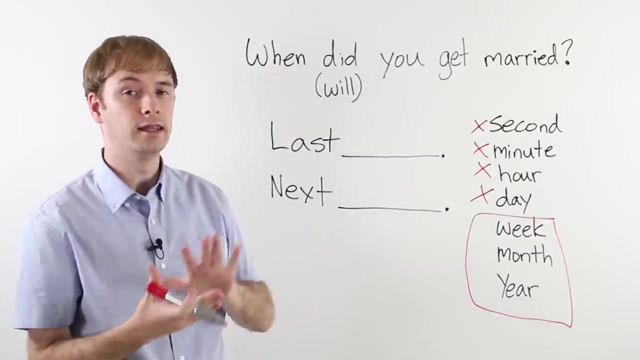 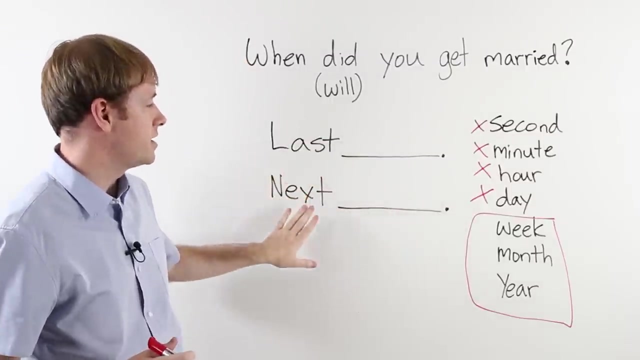 last minute. No, We can't use minute And actually we can't use hour and we can't use day, We can only use these expressions. Ok, so for these ones you want to use ago and later, only Now. these ones you can use ago and later and last and next. Ok, so again. 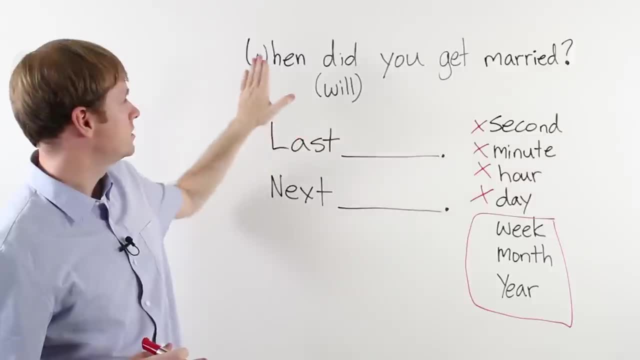 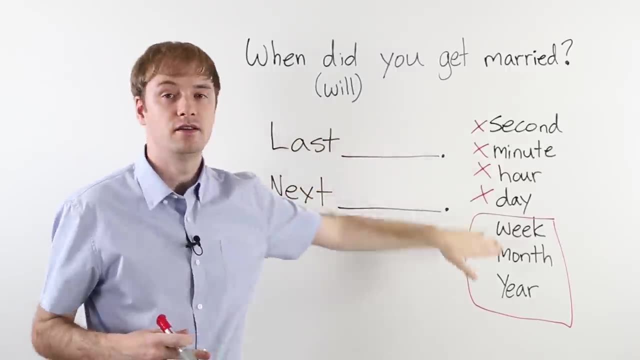 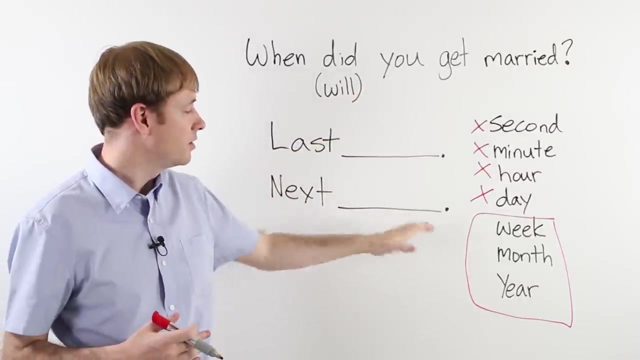 you can't use these with last and next, So let's take a look. When did you get married? Last week, Last month, Last year? Very easy, When will you get married Next week, Next month, Next year? Ok, 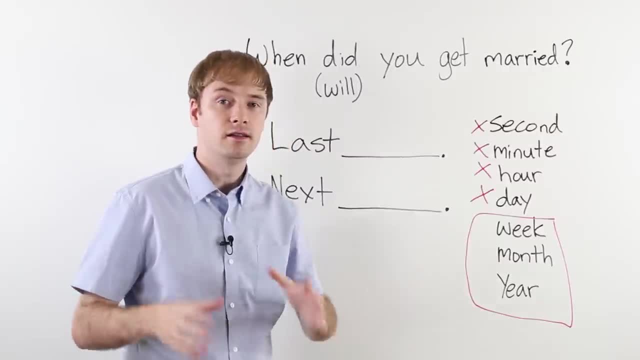 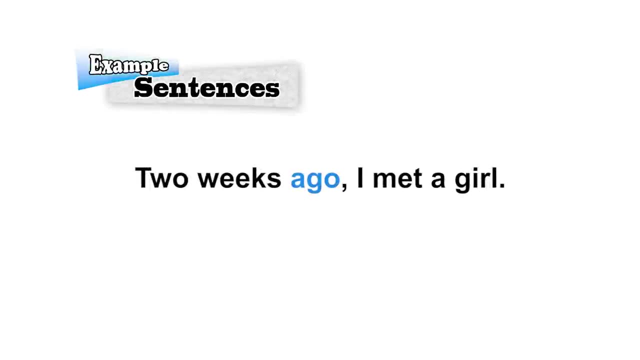 So that's how you use last and next: Very easy. Let's take a look at some examples. Alright, let's look at some example sentences. Listen carefully: Two weeks ago, I met a girl. Two weeks ago, I met a girl. 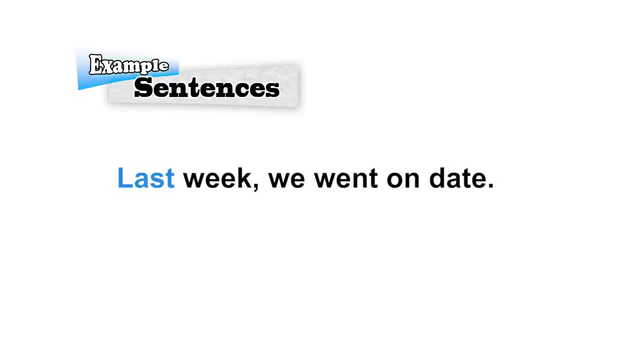 Last week we went on a date. Last week we went on a date Ten minutes ago. I asked her to marry me. Ten minutes ago, I asked her to marry me Two hours later. we will go home. Two hours later, we will go home. 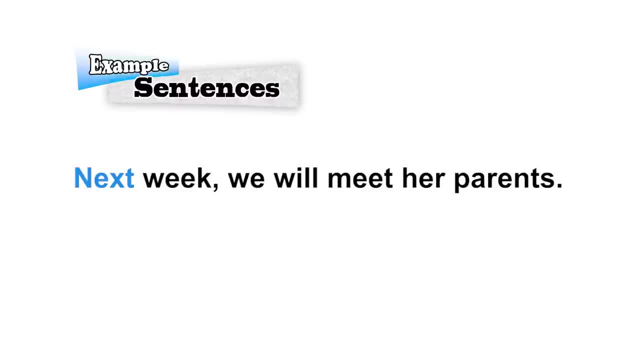 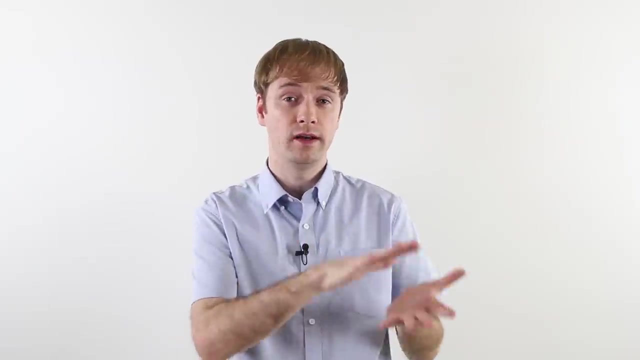 Next week we will meet her parents. Next week, we will meet her parents. Two months later, we will get married. Two months later, we will get married. Ok, I hope you have a good understanding of how to use the time expressions ago and later. 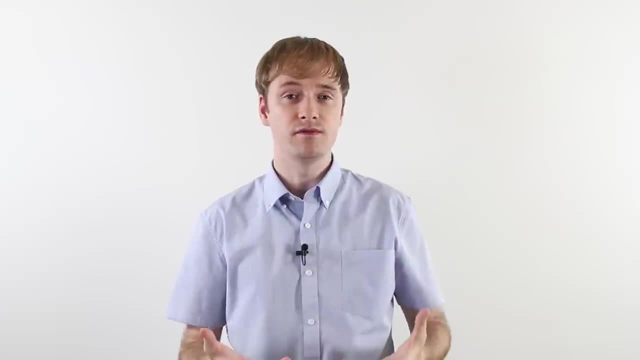 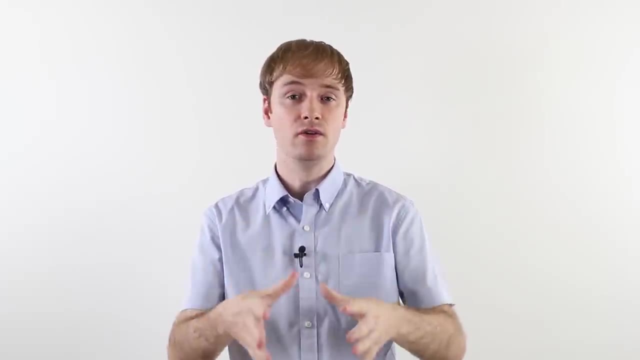 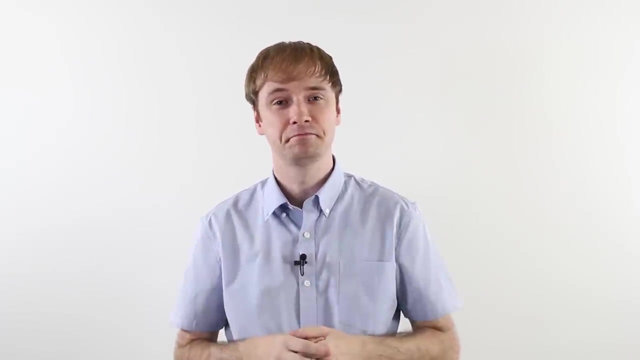 and last and next, They're very useful to quickly express time. alright, So you should study those Self-study. I know you can learn them, I know you can use them, So I hope this video helped you. See you next time. 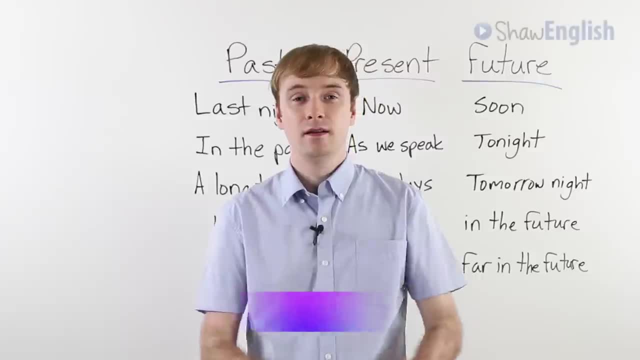 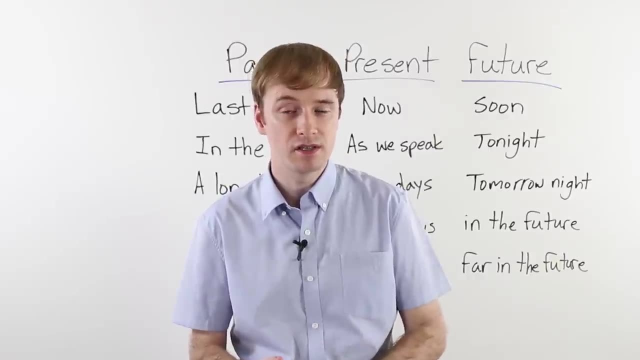 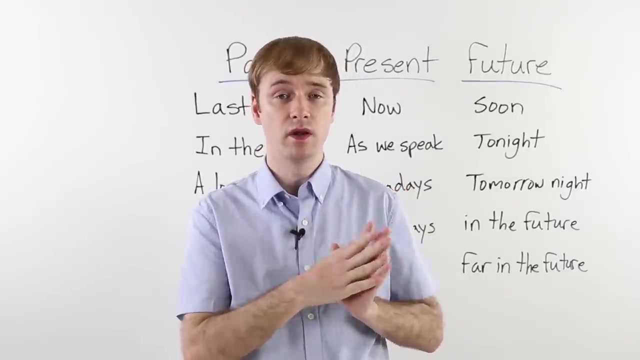 Hello everyone, Welcome to this time expressions video. In this video we're going to talk about time expressions For the past, present and future. Now, in the previous video, the before video, we already studied ago. later, last and next. 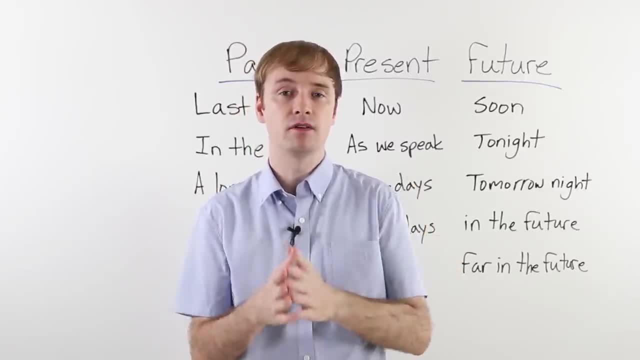 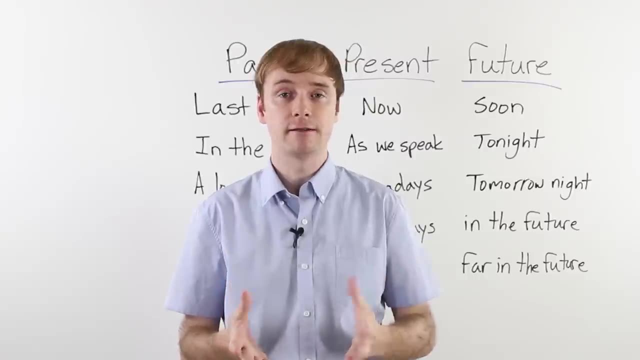 Those ones are common And here are a few more. ok, Now, there's a lot of time expressions, and I can't teach them all, but I tried to choose the most common, Alright, so let's take a look. The first is the past. 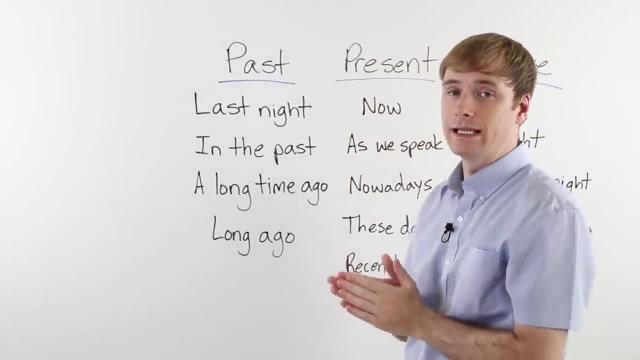 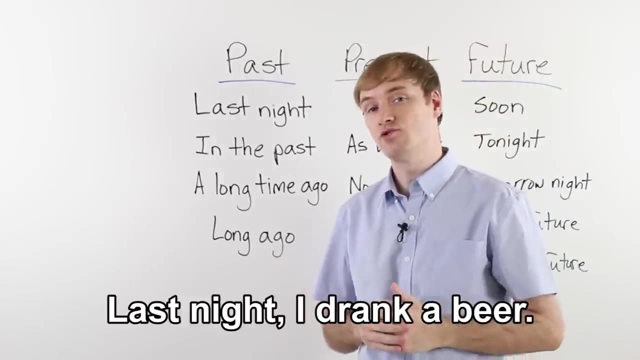 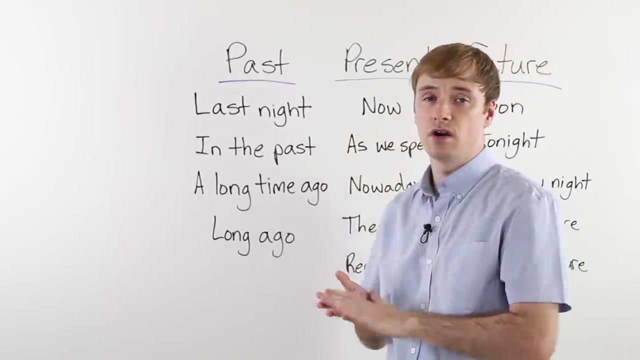 Things that happened before, And the first one very common: Last night, Very easy to use. Last night I ate pizza. Last night I drank a beer. Last night I went to bed early, alright, So very easy to use to talk about yesterday night. 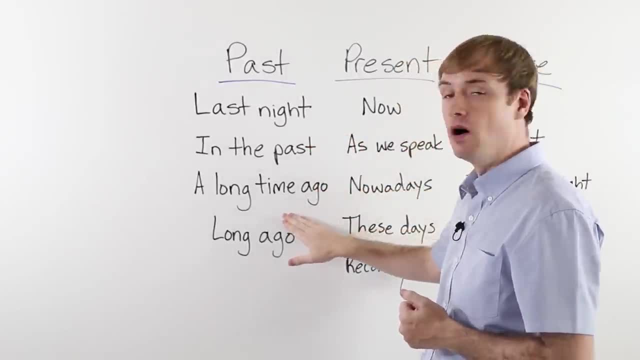 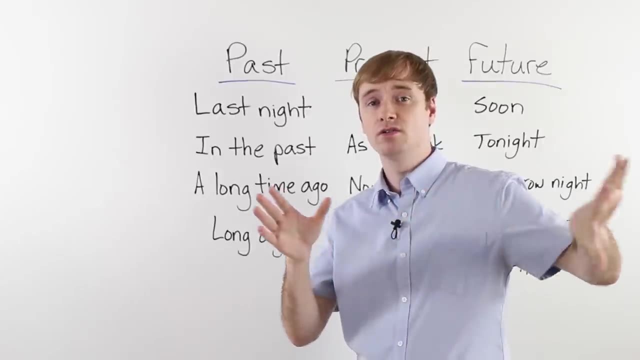 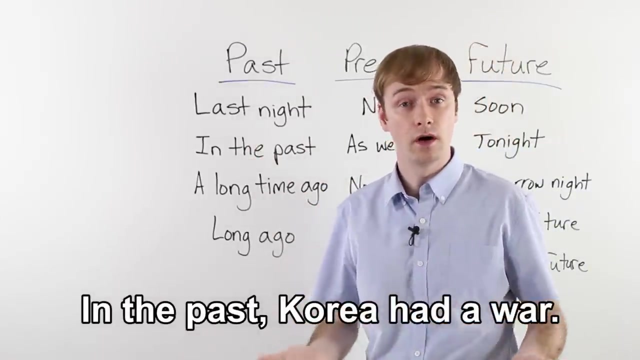 Now the next three. in the past, a long time ago and long ago. ok, These are things that happened before, But a very long time ago, Time has passed. So, for example, in the past, Korea had a war, ok. 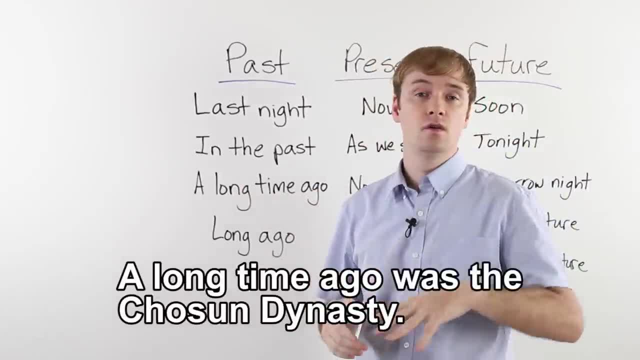 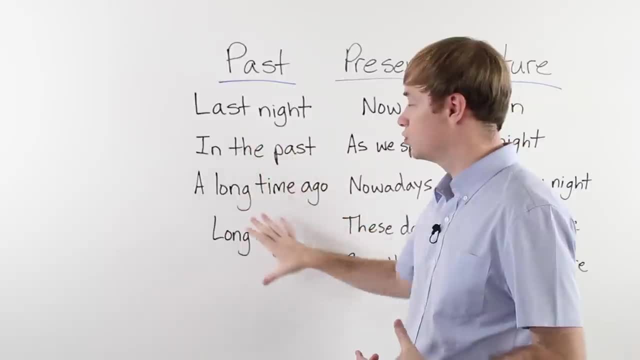 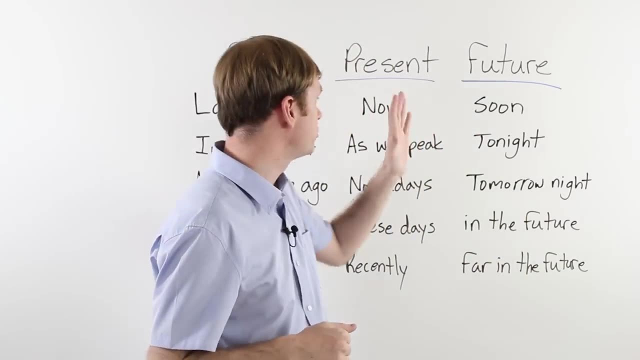 So that was long ago. A long time ago was the Chosun Dynasty? ok, Long ago was the Chosun Dynasty. All of these are good expressions to talk about something long ago. Ok, let's move on to the present. 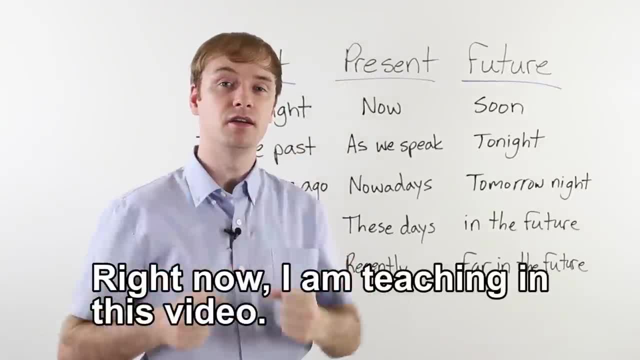 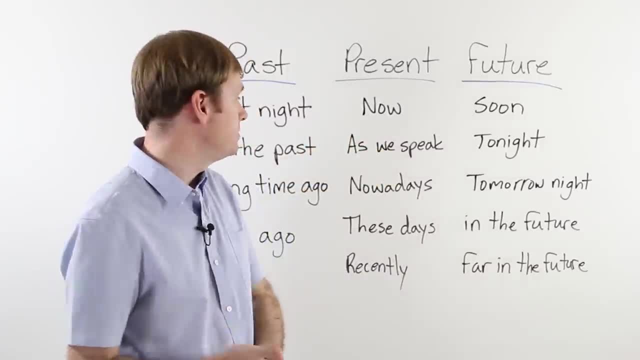 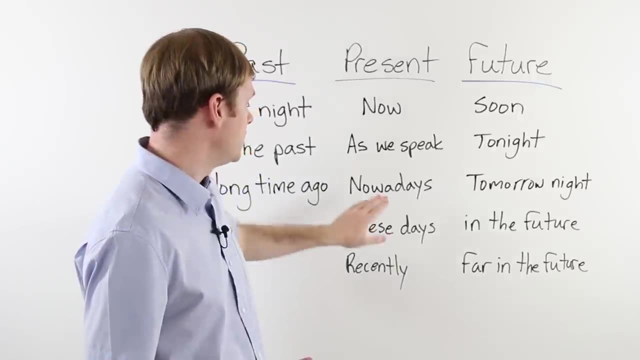 Now, Right now, Right now, I'm teaching in this video Also. we could use this one As we speak. As we speak means the same as now, As we speak. I am teaching this video Nowadays, These days, recently. 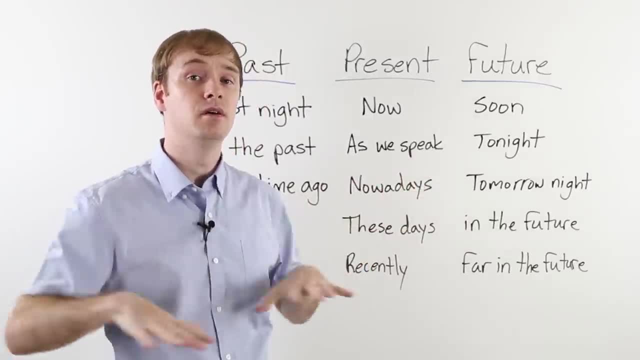 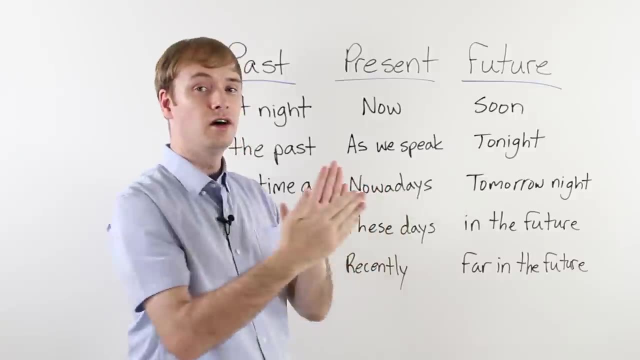 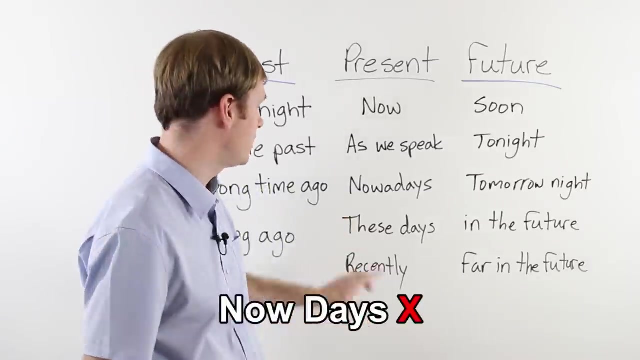 All of these mean the same thing. So something has happened around this time. Now be careful with nowadays. Nowadays is one word A lot of my students say. nowadays, Nowadays is wrong. Don't say nowadays, You have to say now-a. 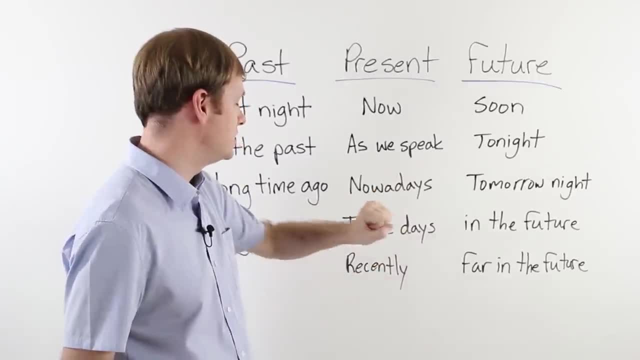 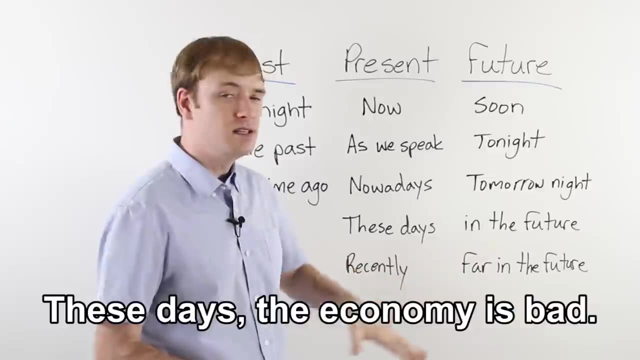 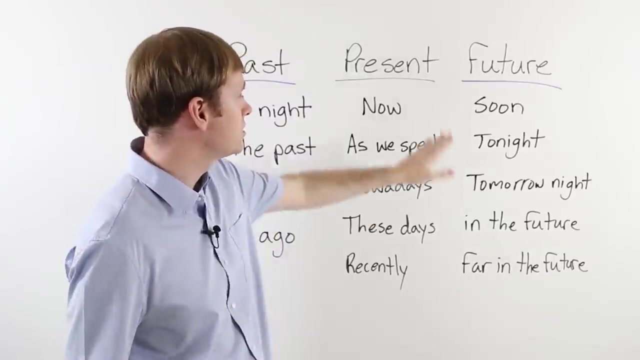 There's an A there Nowadays, Nowadays, These days, Recently. So nowadays the weather is very hot, Or these days the economy is bad. alright, So all of them very similar. Alright, let's go to the future, Soon. 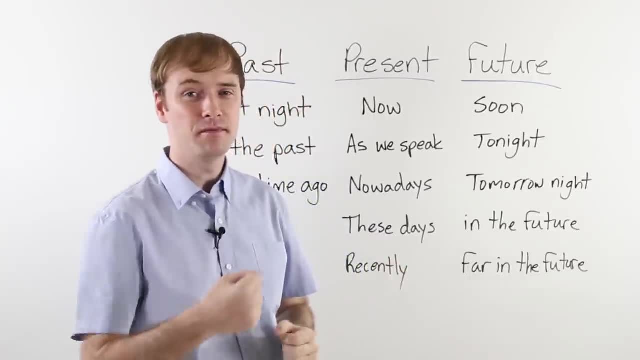 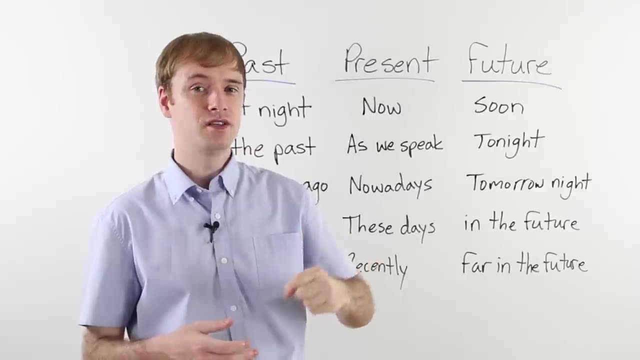 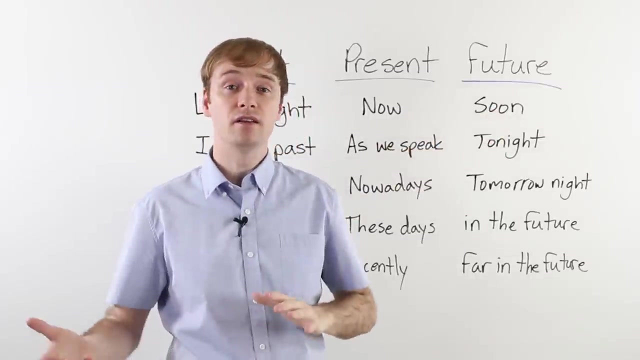 A lot of my students like to say coming soon, Coming soon. Now we usually use coming soon for movies that are coming soon, But just when we're talking with our friends we don't usually say coming soon. We say soon, My friend is coming soon. 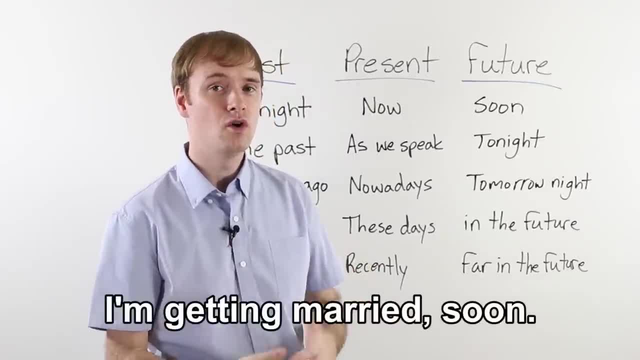 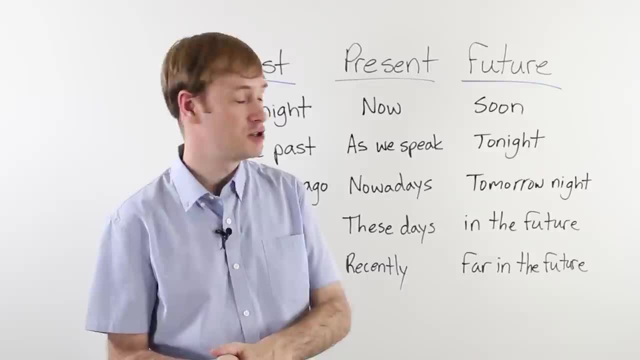 That's okay, But I'm getting married soon Or I'm going to eat dinner soon. Okay, I'm going to use it like that. Don't use coming soon, Too soon, Too much Tonight. Tonight I'm going to have a good dinner. 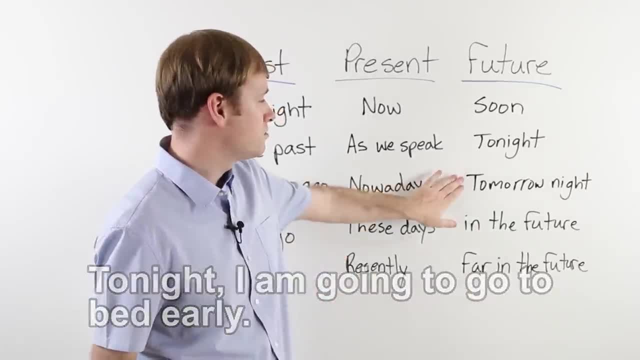 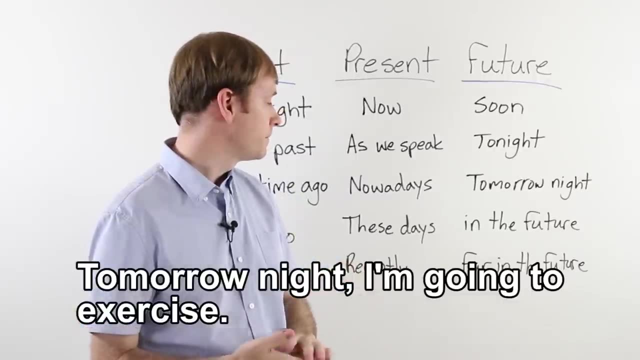 Tonight I'm going to go to bed early. Tomorrow night, Okay, Tomorrow night I have to meet my friends. Tomorrow night I'm going to exercise, Alright, And the last two In the future, Far in the future. 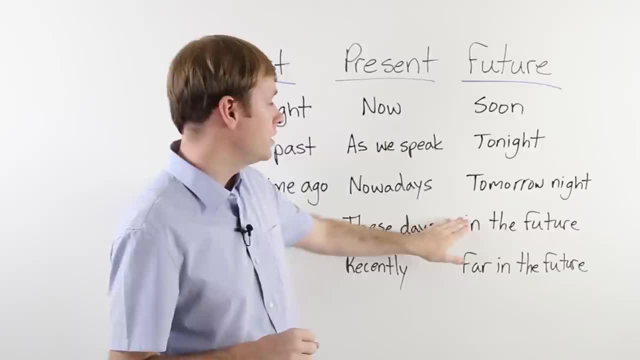 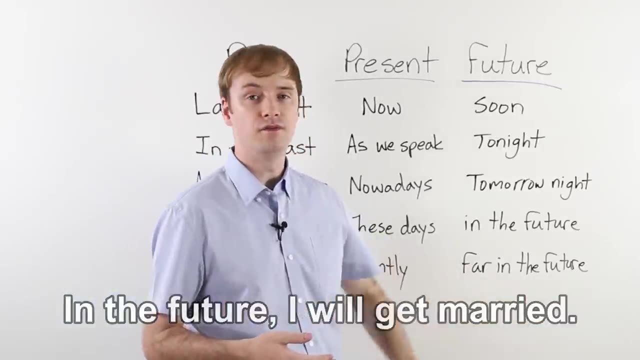 Alright. So we're talking about a long time. So in the future- I don't know when In the future- I will get married, Alright, Far in the future. Far in the future, maybe twenty years later I will retire. 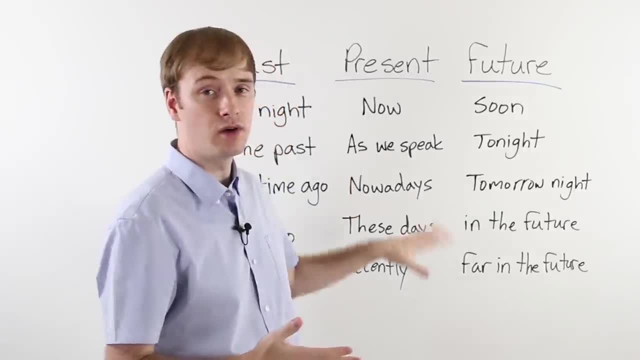 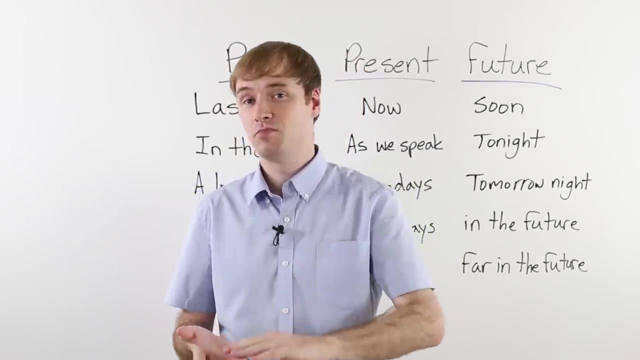 I will quit my job Alright, So I'm sorry I had to go a little bit quick through these expressions. These are good time expressions to express past, present and future. Let's take a look at a few examples right now. 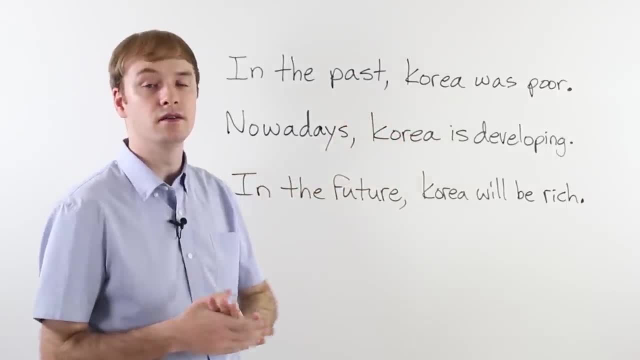 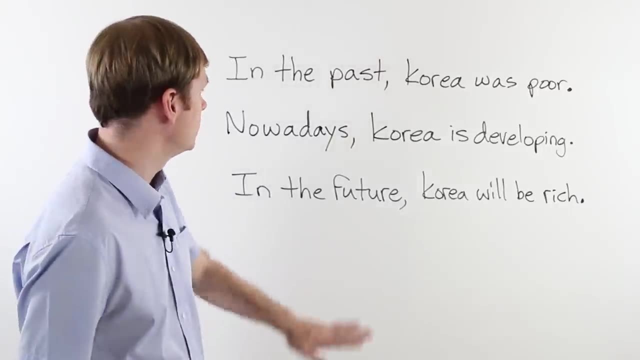 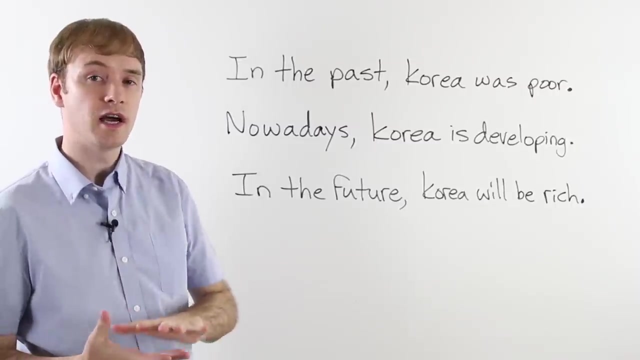 Okay, I wrote three sentences here to help you understand How to use the time expressions: past, present and future. Let's take a look at the first one: In the past. Okay, We should try and always use our time expression at the beginning of the sentence. 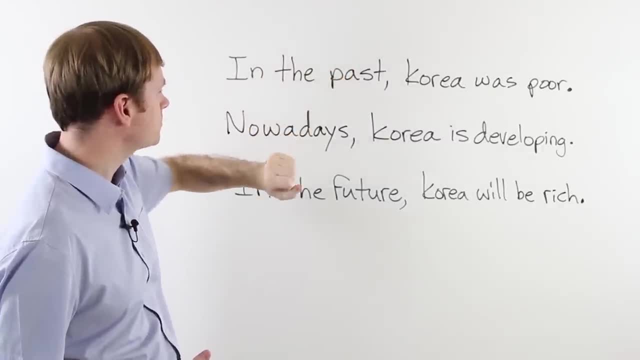 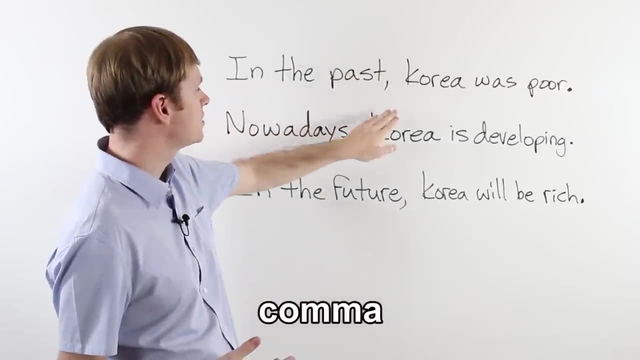 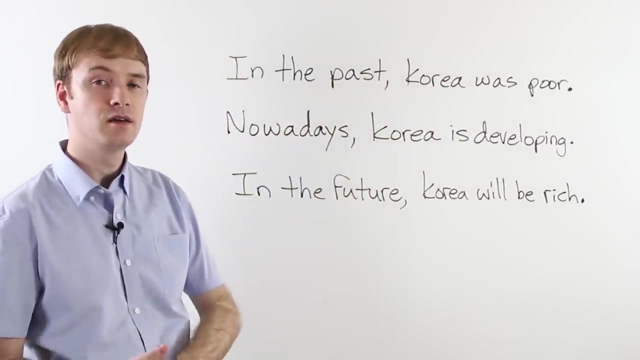 So in the past. that's my time expression. After our time expression, we should use a comma In the past comma. So In the past, Korea was poor. In the past Korea was poor. Alright, The economy was not good. 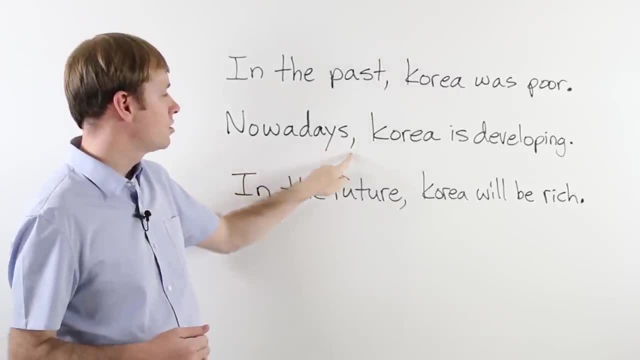 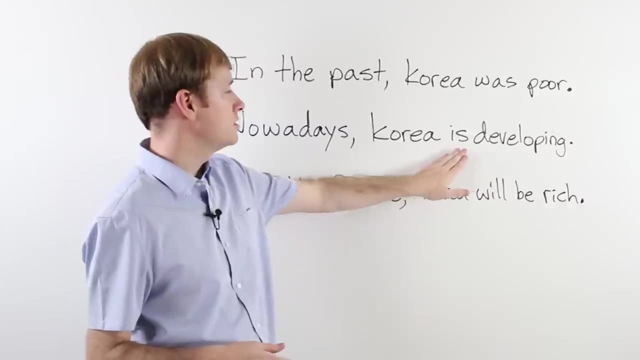 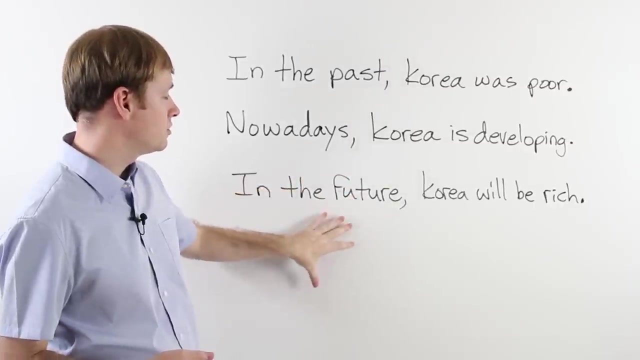 Let's look at the next sentence: Nowadays, comma. So nowadays, these days, recently, Korea is developing. Okay, nowadays, Korea is developing. Again, I have a comma. And let's go to the future. In the future, Korea will be rich. 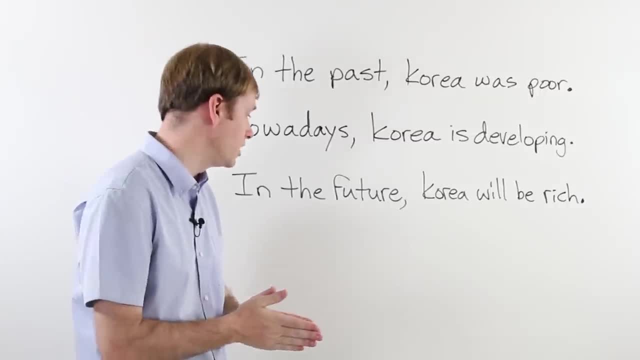 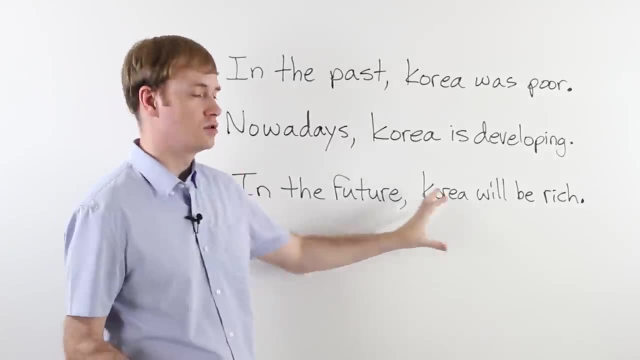 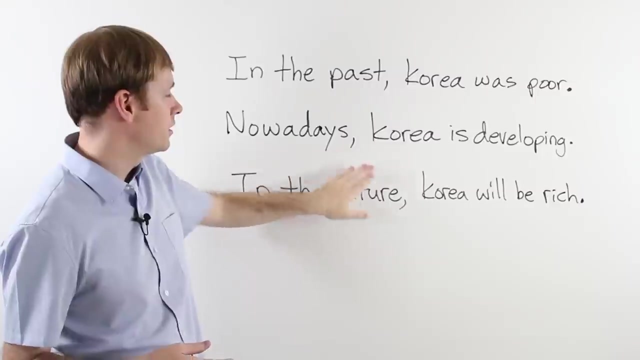 In the future, Korea will be rich In the future, far in the future, soon, Maybe soon, Soon, Korea will be rich, Okay. So again, use the time expressions in the beginning, followed by a comma there. Okay. 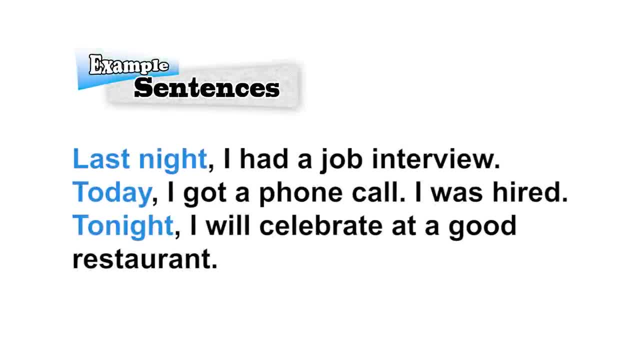 So let's look at some more examples. Example one: Last night I had a job. I had a job interview. Today I got a phone call. I was hired. Tonight I will celebrate at a good restaurant, Okay. example number two: 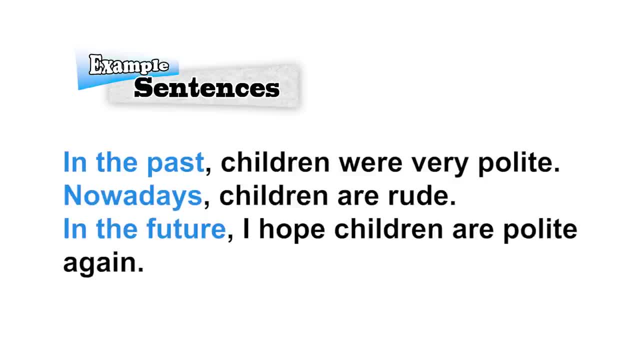 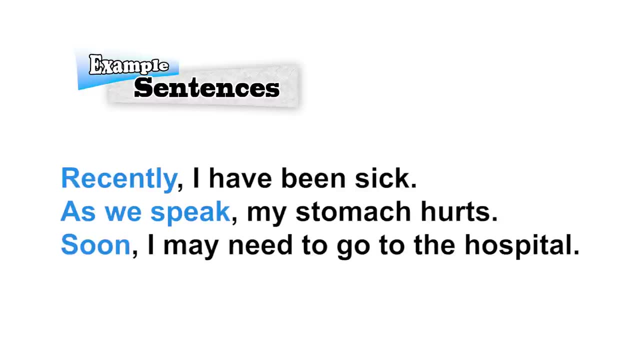 In the past children were very polite. Nowadays children are rude. In the future, I hope children are polite again Right Next example: Recently I have been sick As we speak. my stomach hurts. Soon I may need to go to the hospital. 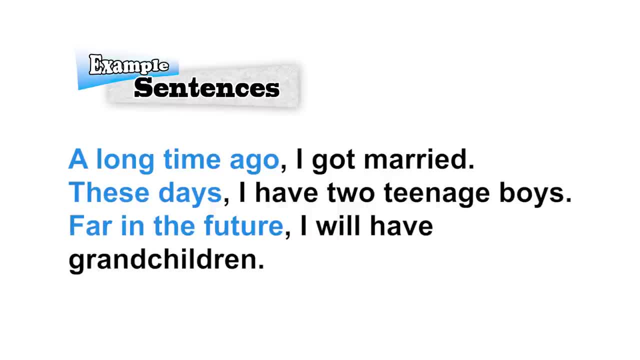 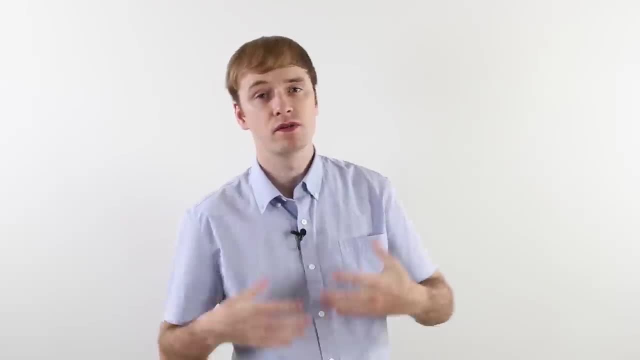 Alright, the last example: A long time ago, I got married. These days, I have two teenage boys. Far in the future, I will have grandchildren. Okay. So here's the example: grandchildren, okay. so those were some good examples of how to use the time. 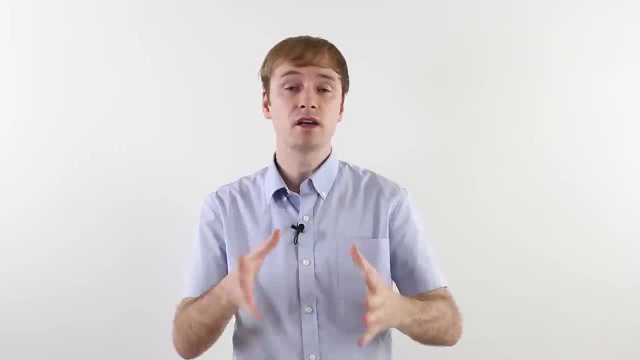 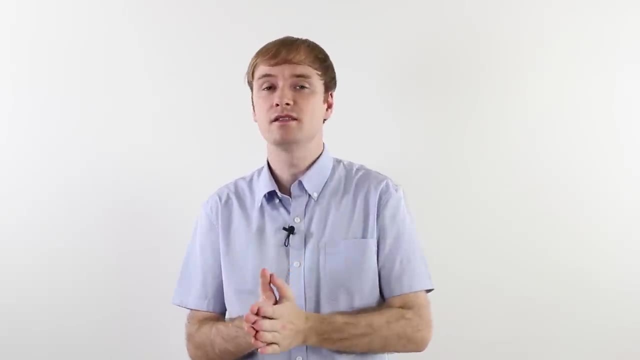 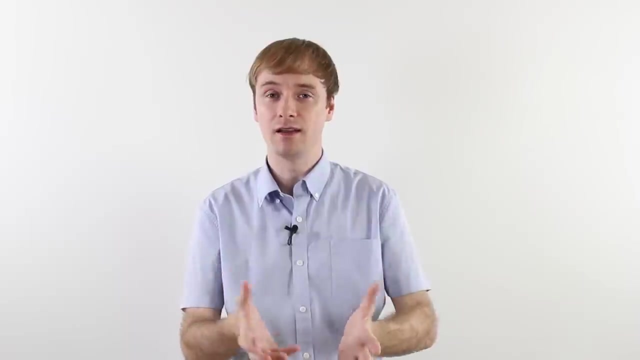 expressions of past, present and future. now, as I taught you, you should try and use the time expressions at the beginning of the sentence, but in some cases it is okay to use them at the end. all right, that's. that's not a bad thing. anyway, I hope you understand. I know there's a lot to learn in this video. I 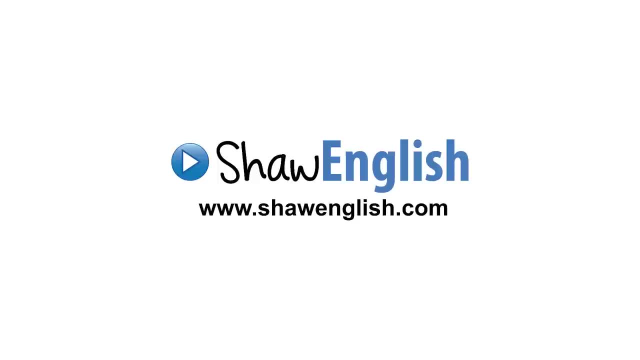 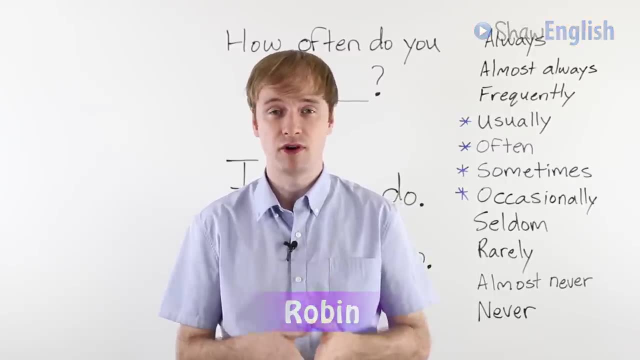 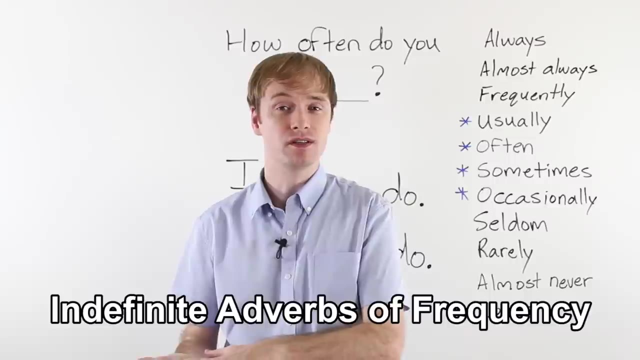 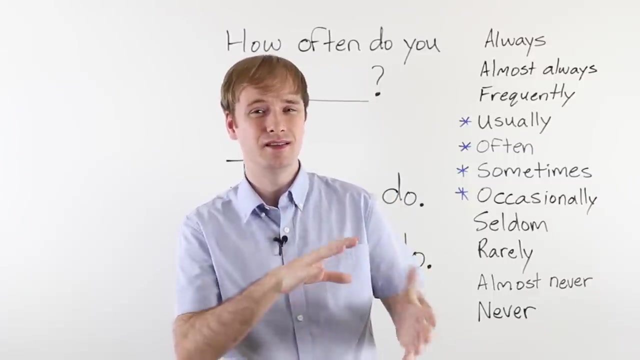 hope to see you again soon. hello everyone, welcome to this time. expressions video. in this video we are going to talk about indefinite adverbs of frequency. okay, what are indefinite adverbs of frequency? well, indefinite means the time is not exact, not detailed, and adverbs of frequency are not exact. and adverbs of frequency are not exact and adverbs of 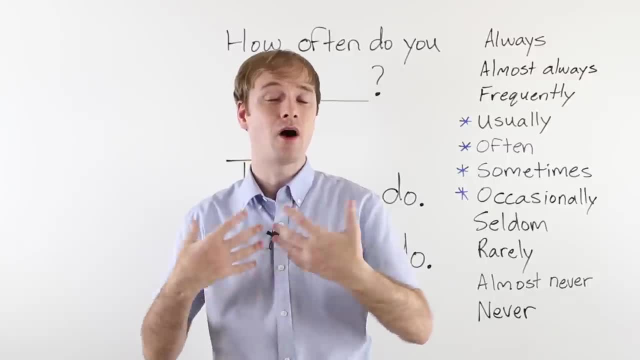 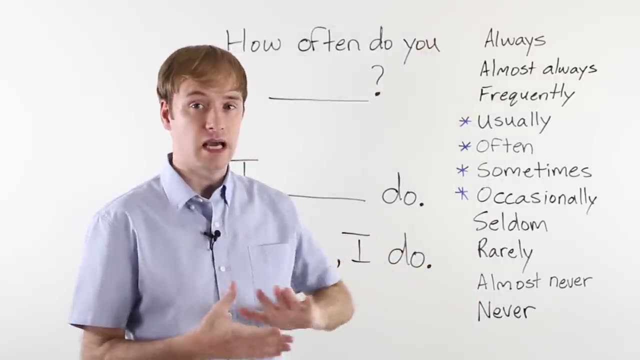 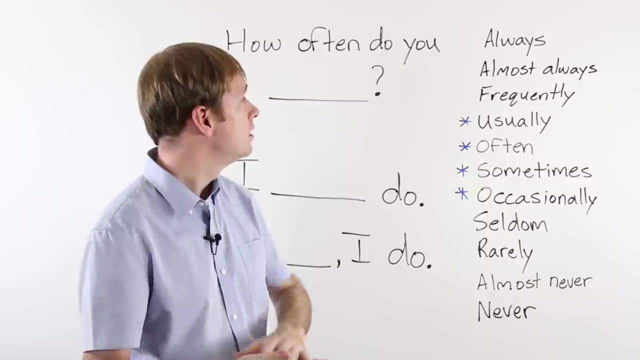 frequency are not exact and adverbs of frequency are words that describe how often we do something. okay, so to help you understand, let's look at the list of adverbs of frequency. these are the most common, all right? so how often you do something? let's go through the list. of course, the top one is always. that means: 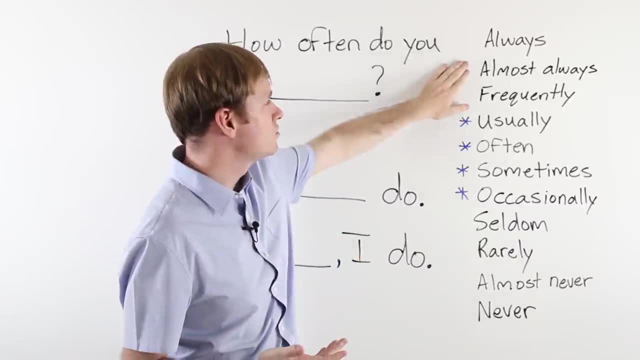 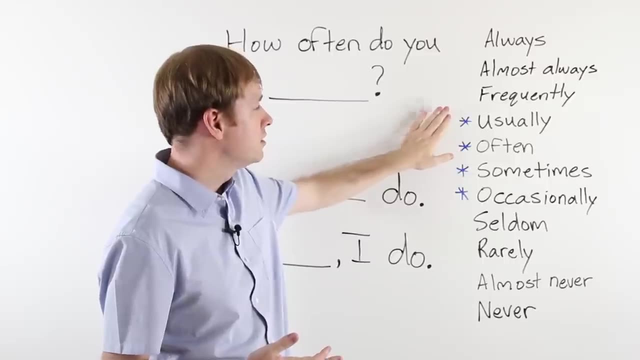 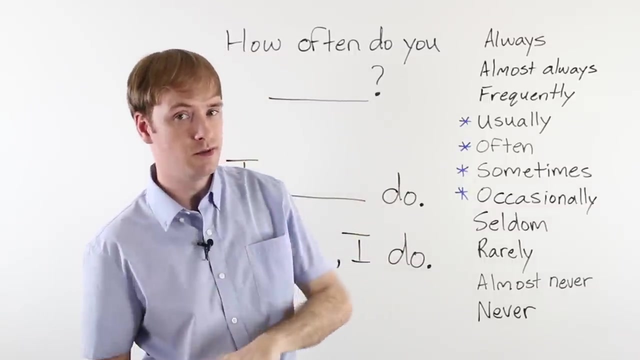 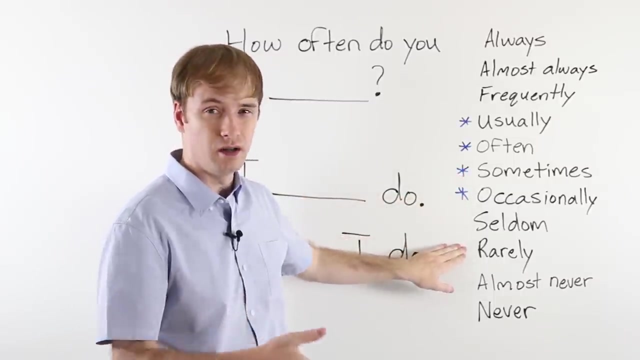 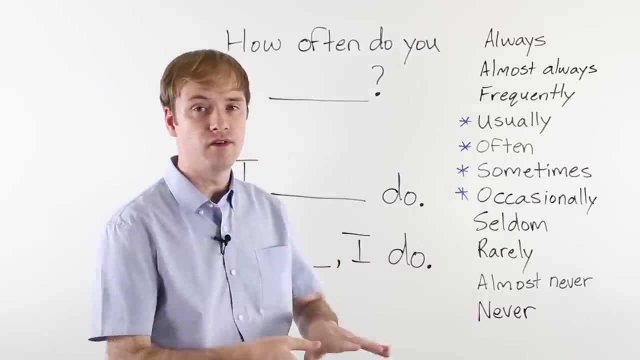 you always do something, almost always very close, frequently, okay, you do it a lot usually, often, sometimes, okay, sometimes is the middle. so sometimes you do something, sometimes you don't. occasionally, occasionally, seldom, rarely, okay, you don't do something very much, almost never. and the last one: never. you never do something, okay. so let's look at our question this: 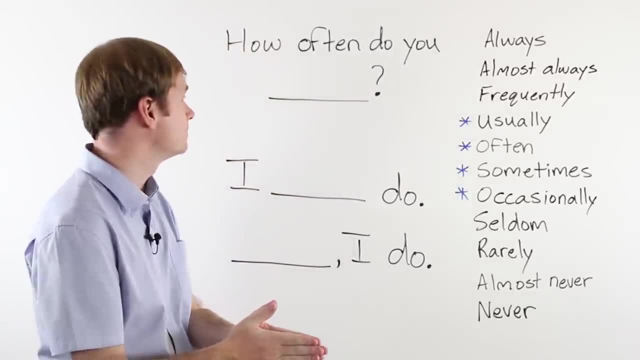 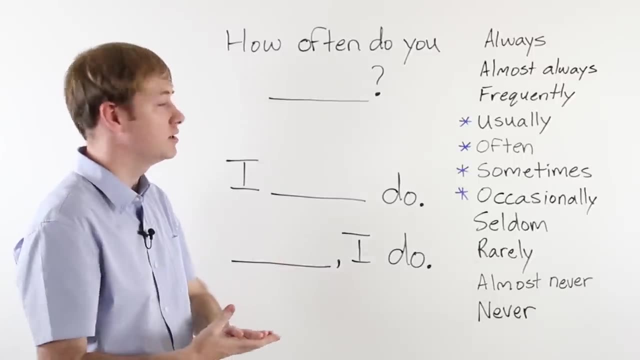 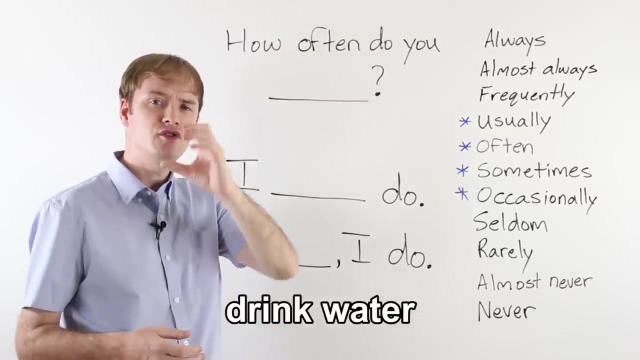 is the important question we want to answer: how often? how often do you so? how often do you do something? so let's make an example question: how often do you drink water? okay, how often do you drink water? so someone asks you that question: how often do you drink water? 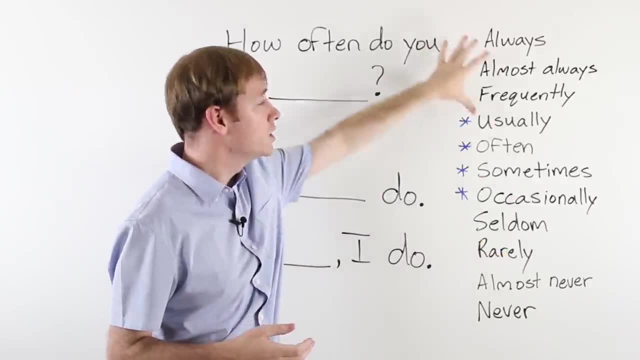 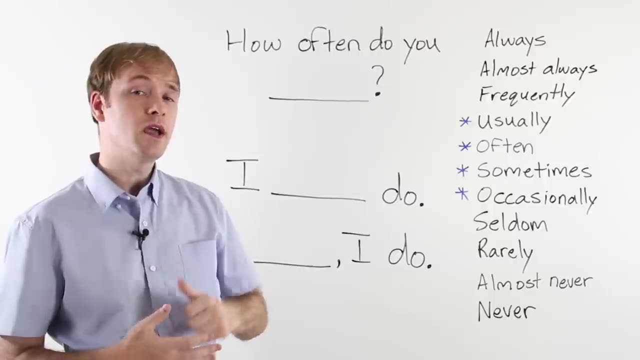 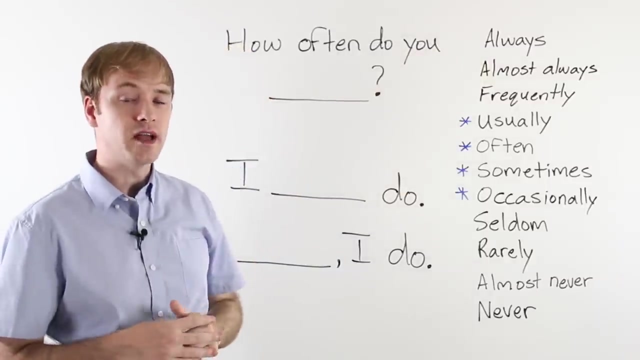 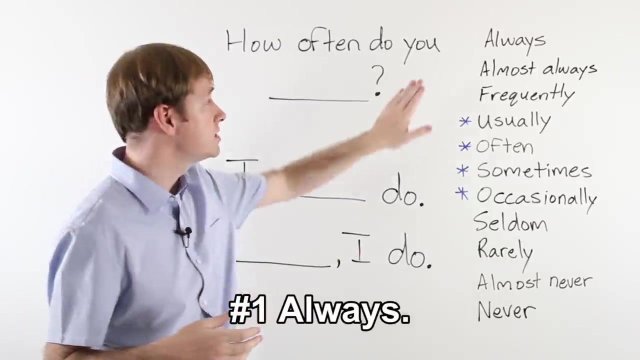 okay. so first you should think about which one of these describes how often you drink water. so there's actually three ways to answer this question. now I'm going to choose always. so the first way to answer- how often do you drink water- I would say always. okay, very simple. you just say the adverb of frequency. how? 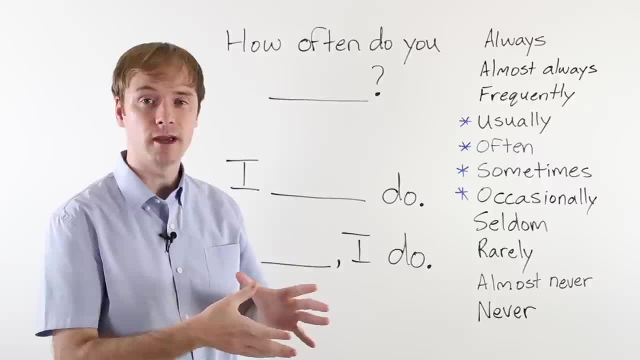 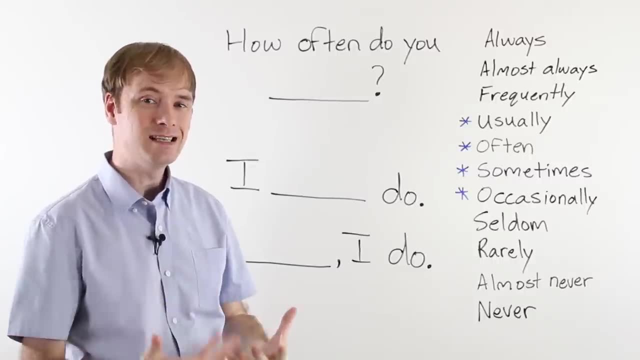 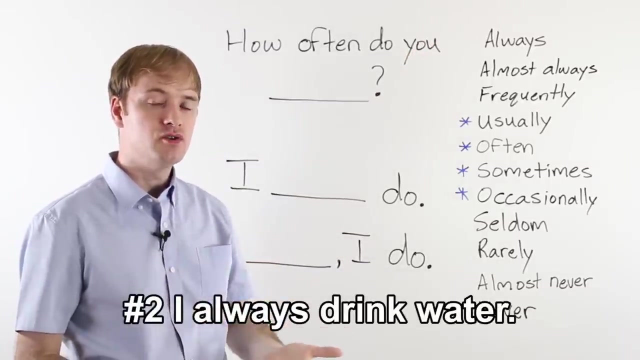 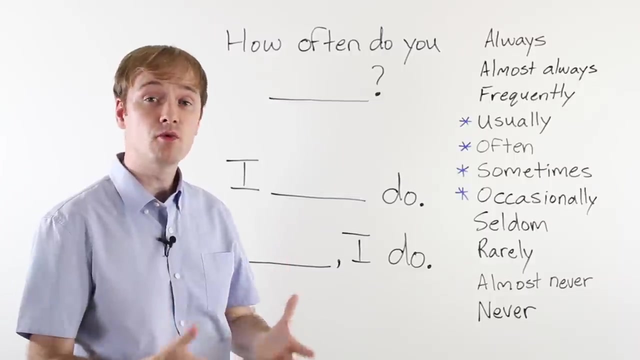 often do you drink water? always, okay, that's the easiest way. the second way: how often do you drink water? okay, you would use a complete sentence, a full sentence. I always drink water. how often do you drink water? I always drink water, all right. and the last way, which is probably the most common way, is this: 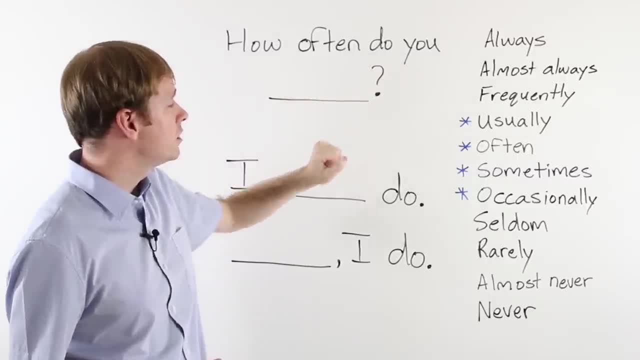 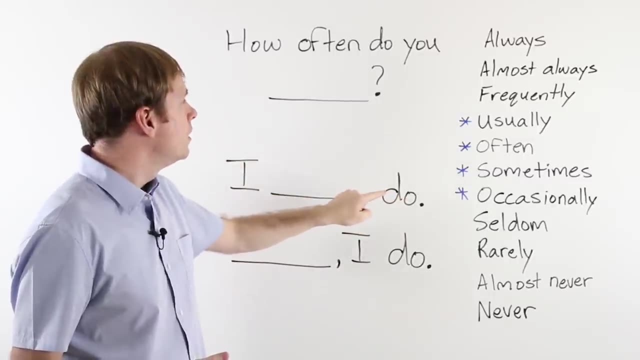 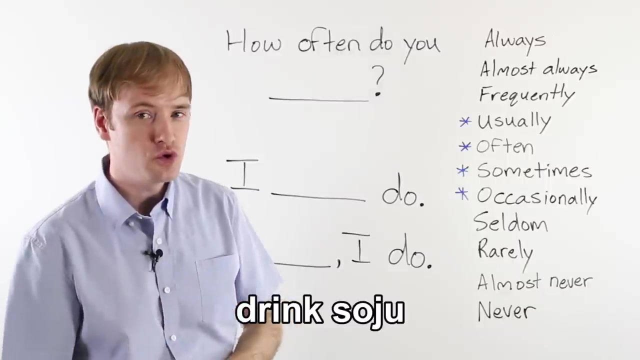 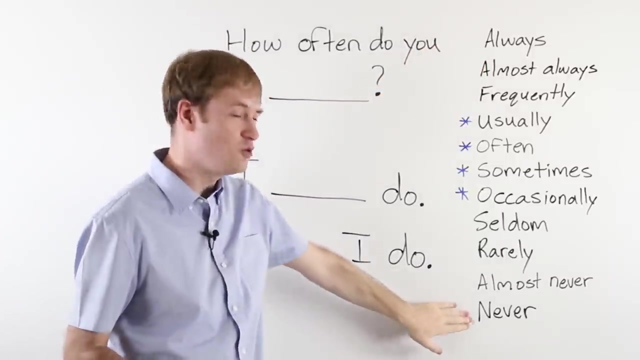 one here: how often do you drink water? I always do. okay, I always do. this is a good sentence to use. all right, let's change the question. how often do you drink soju? okay, how often do you drink soju? some of you are always, some of you are never. I'm gonna choose sometimes, so I'm gonna say I. 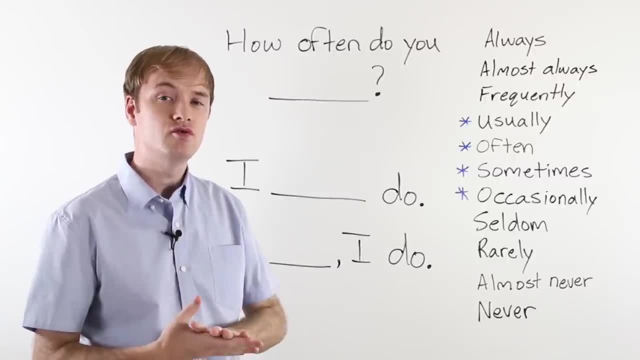 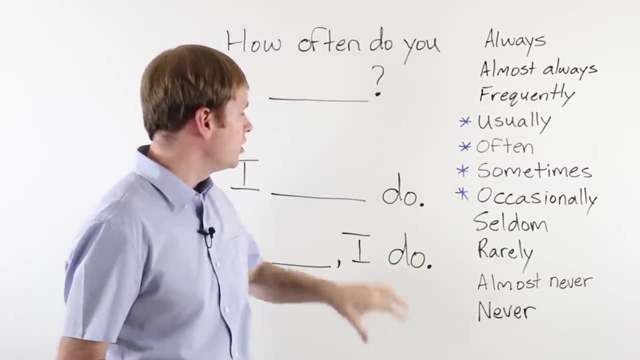 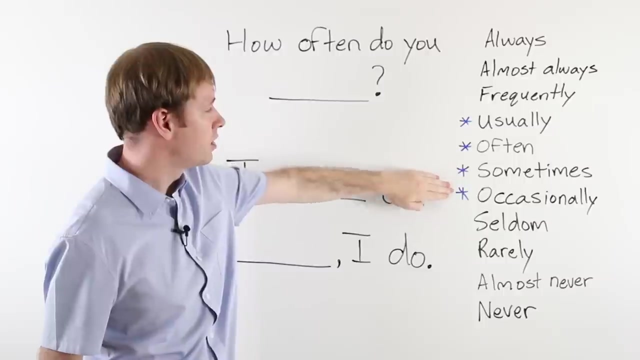 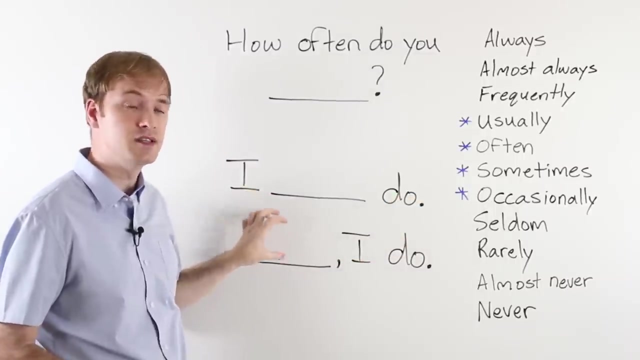 sometimes do. how often do you drink soju? I sometimes do. all right now, the adverbs of frequency are usually in the middle of the sentence. Ok, but you see these ones here with the star. These ones are in the middle, but also we could use them at the beginning of the sentence. 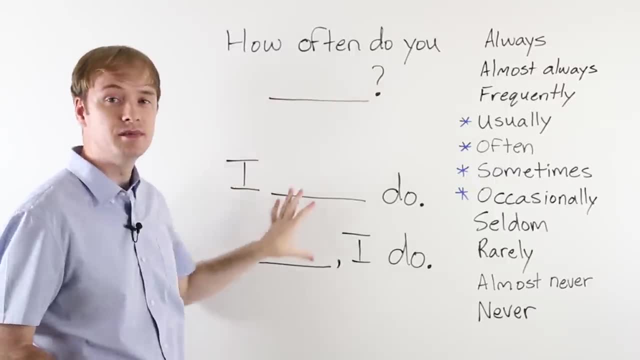 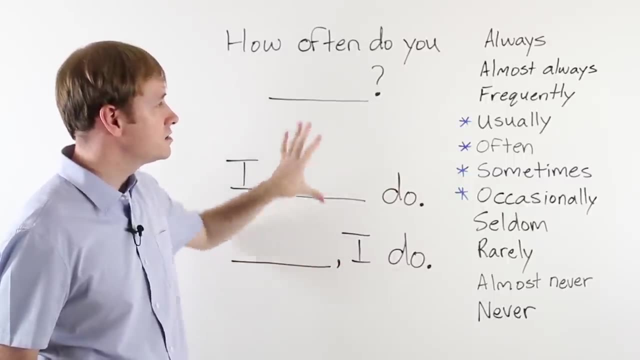 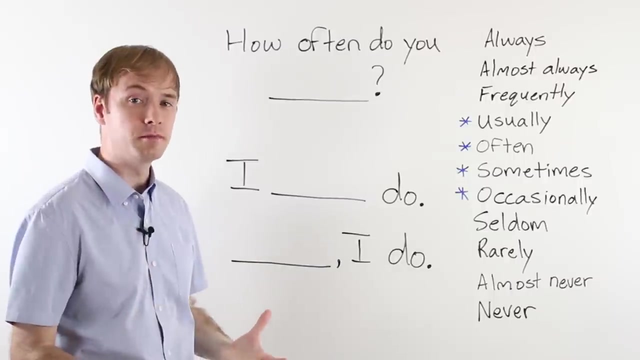 So how often do you drink soju? Sometimes I do, I sometimes do. Both ways are ok Alright. so these are the adverbs of frequency. I know it takes a lot of practice to remember them and use them properly, So we're going to look at a few more examples right now to help you understand them. 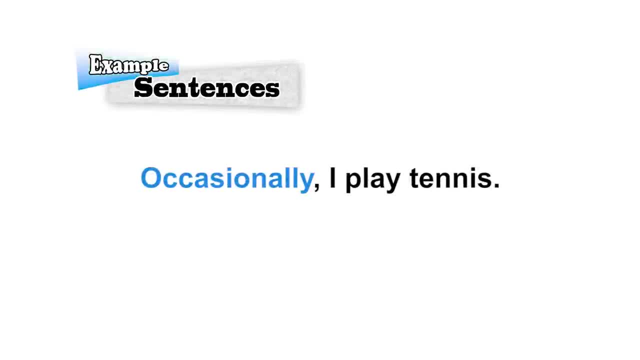 Ok, let's look at some example sentences. The first one: Occasionally I play tennis. Occasionally I play tennis. I frequently swim at the beach. I frequently swim at the beach. Sometimes I go fishing. Sometimes I go fishing, I always have a headache. 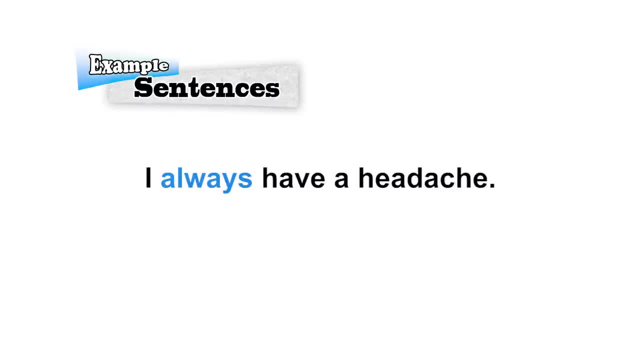 I always have a headache. My wife usually comes home late. My wife usually comes home late. She, She almost never studies. She almost never studies. We hardly ever hold hands. We hardly ever hold hands. They often fight, They often fight. 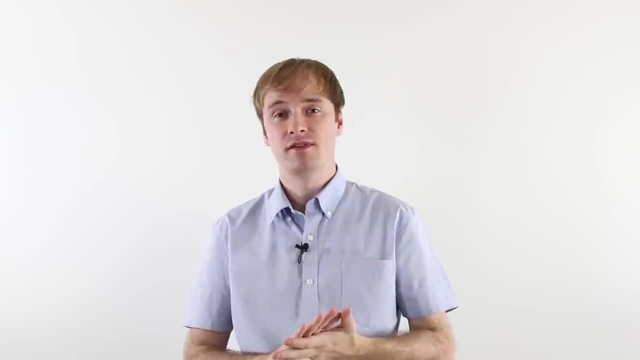 Alright, so those were some good examples of how to use indefinite adverbs of frequency Now. they're very useful to know, so you should study them Now. I couldn't talk about everything in this video, so you need some extra self-study. 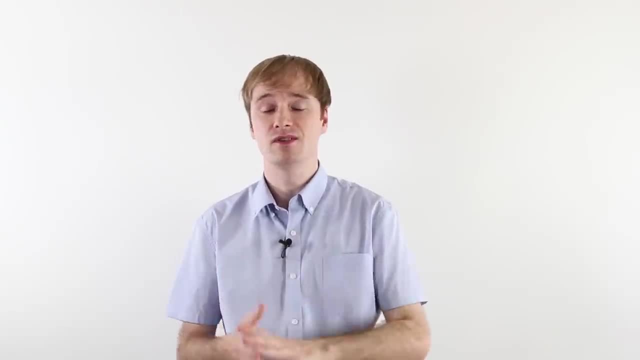 Learn them, Use them. They're very useful to express how often you do something. Alright, so that's it for this video. See you next video. Hello everyone, Welcome to my YouTube channel. I hope you're having a great day. 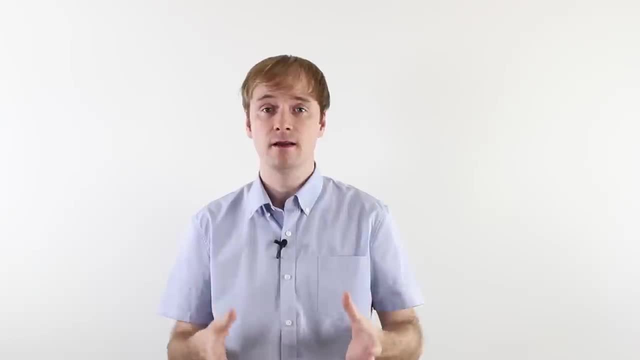 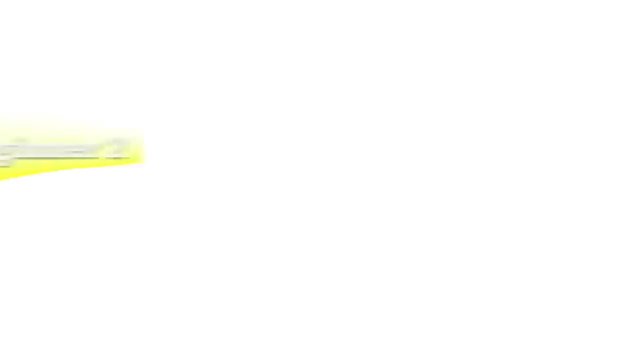 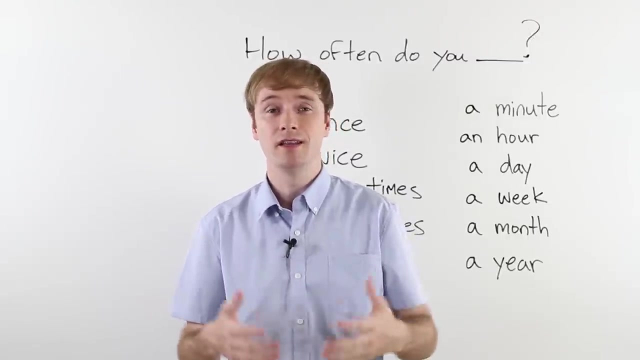 Bye-bye, Bye-bye, Bye-bye, Bye-bye, Bye-bye, Bye-bye, Bye-bye, Hello everyone, Welcome to this time expression video. In this video, we are going to learn how to use definite adverbs of frequency. 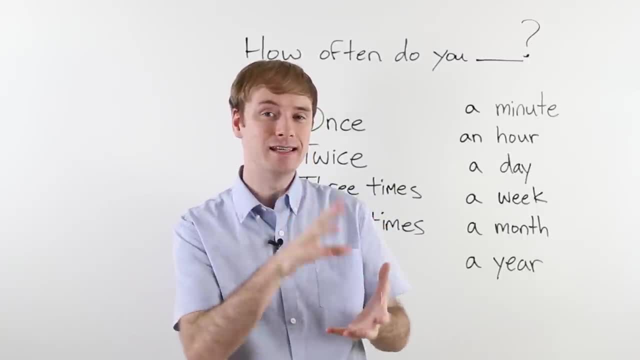 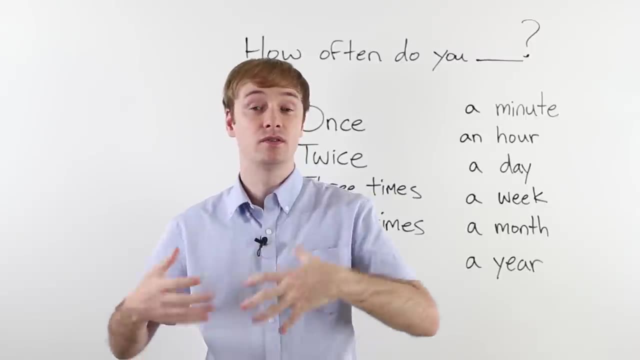 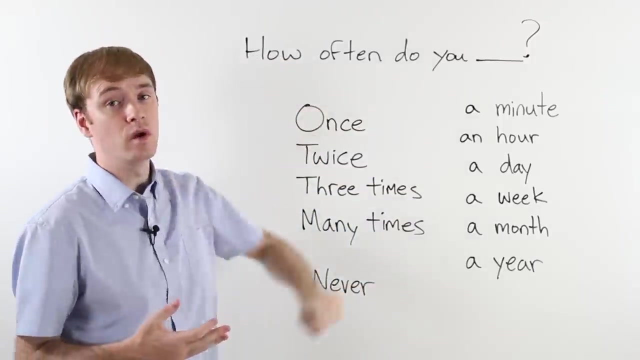 What does that mean? Well, definite means an exact time, an exact amount And the adverbs of frequency. okay, those are words to describe how often we do something. Alright, so let's take a look. This is the question we want to answer. 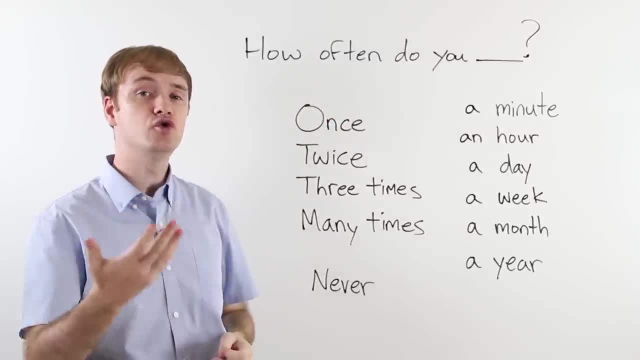 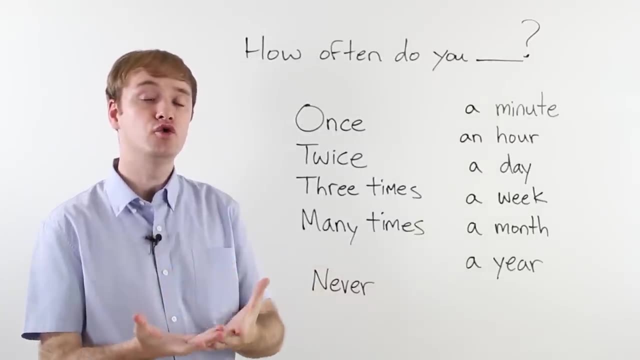 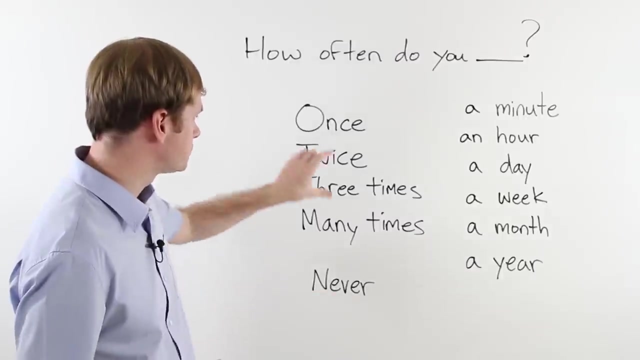 So someone asks: how often do you do something? So let's do an example. I will ask: how often do you take a shower? How often do you take a shower? Okay, so we have to answer Now. let's start with once. 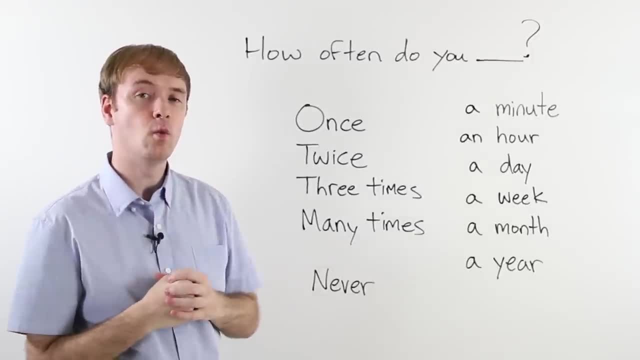 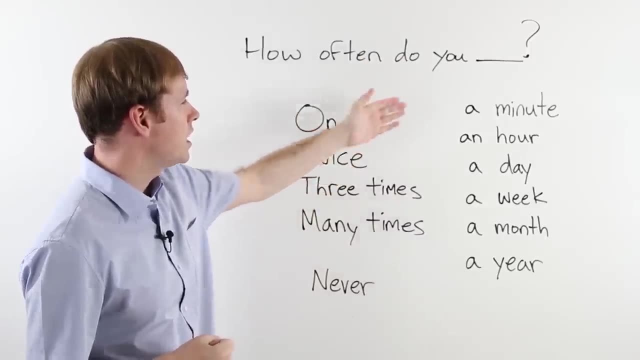 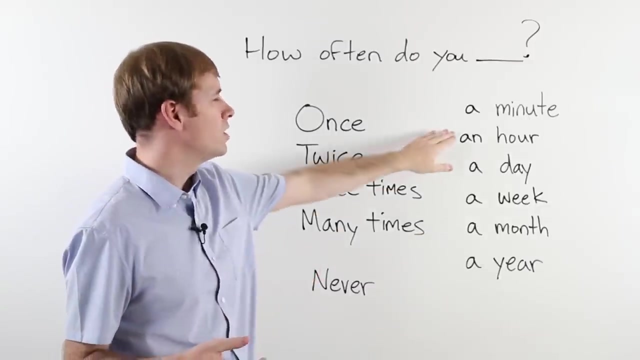 Once means one time, but we don't say one time, We use the word once. So how often do you take a shower Once? and then I would choose one of these. okay, Once a minute, Okay, that's a lot of showers. 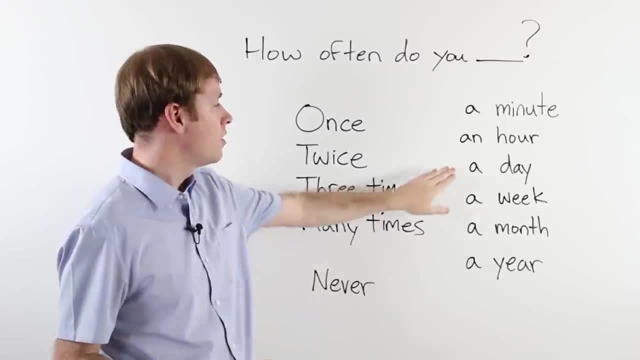 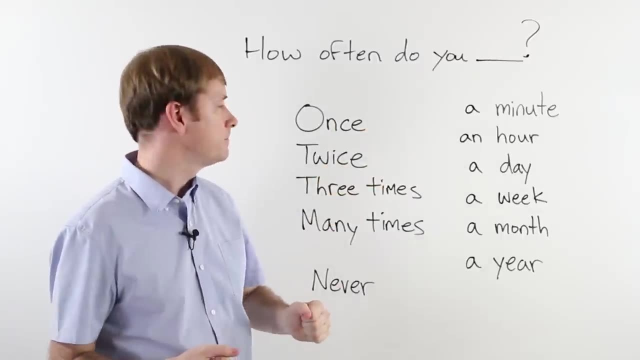 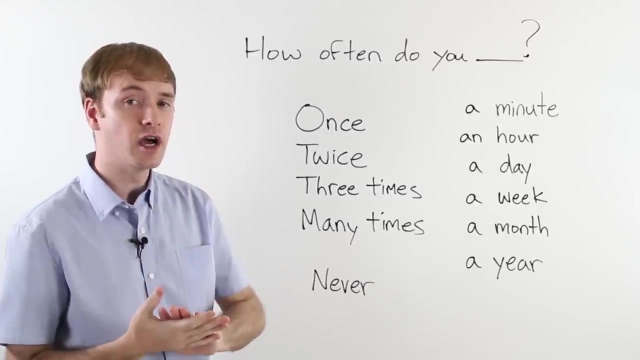 Once an hour. That's still a lot of showers. Once a day? That sounds right. How often do you take a shower Once a day? Alright, Now, some of you maybe you take a shower two times, but we don't say two times. 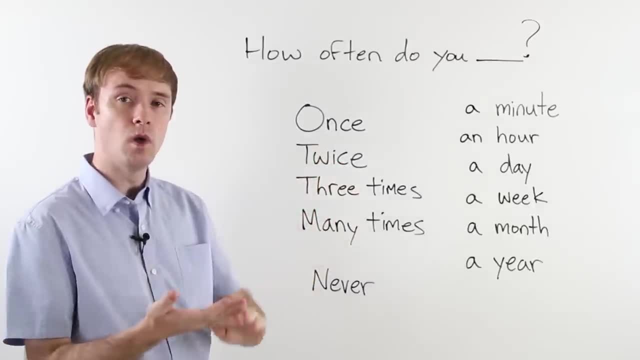 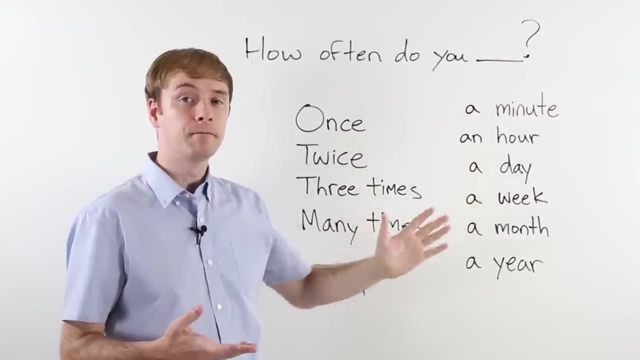 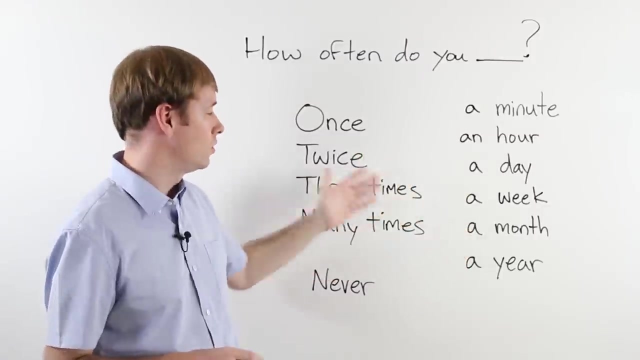 We say twice Okay, So we use once twice. How often do you take a shower? Twice a day, Okay, And if you're a very dirty person, maybe twice a week, twice a month or once a year. That's a very dirty person. 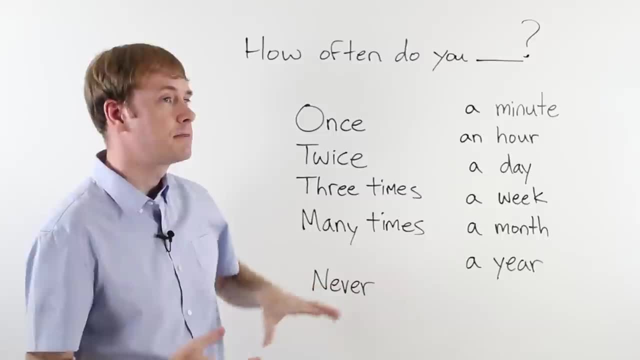 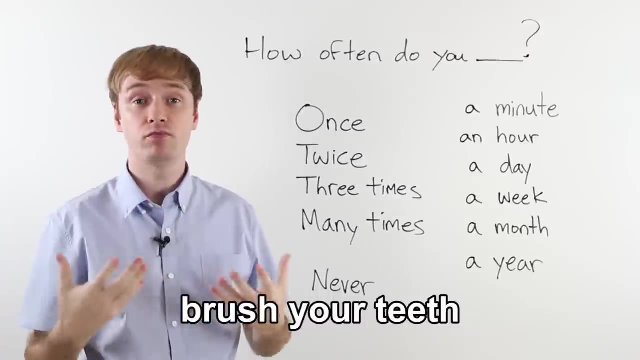 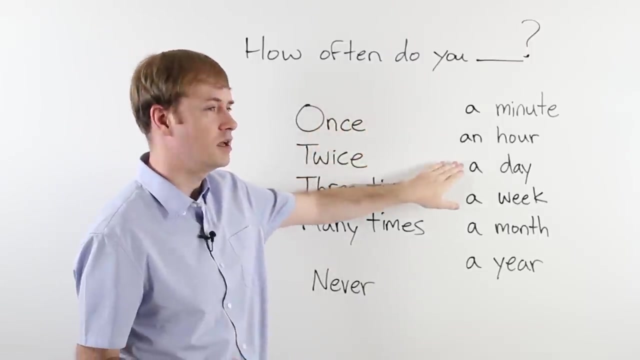 Okay, so we have once twice. I'll change the question: How often do you brush your teeth? How often do you brush your teeth? Well, I brush my teeth. let's see, once a day, no, no, twice, no, I'll say three times. 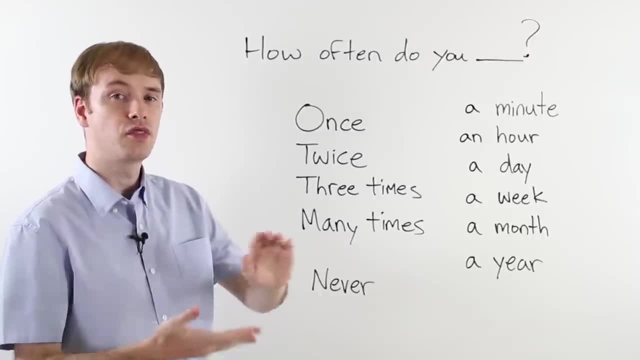 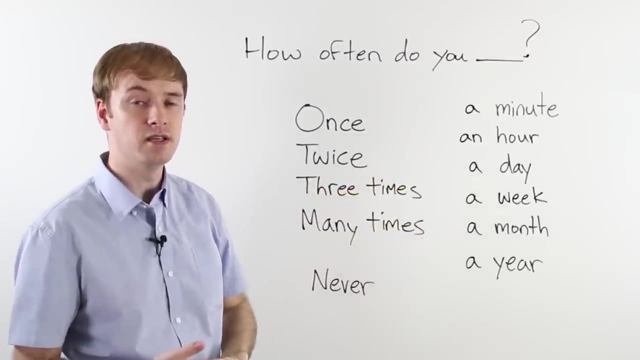 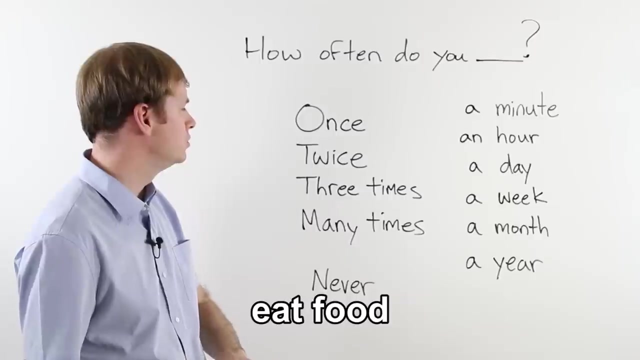 Okay. so we say once, twice, three times: I brush my teeth three times a day, Three times a day. How often do you eat food? Hmm, I eat food three times a day, Three times a day, Three times. 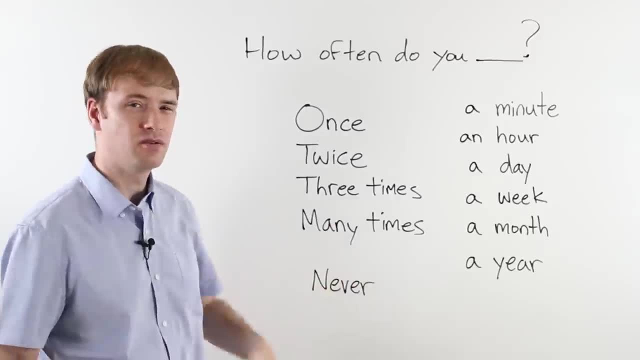 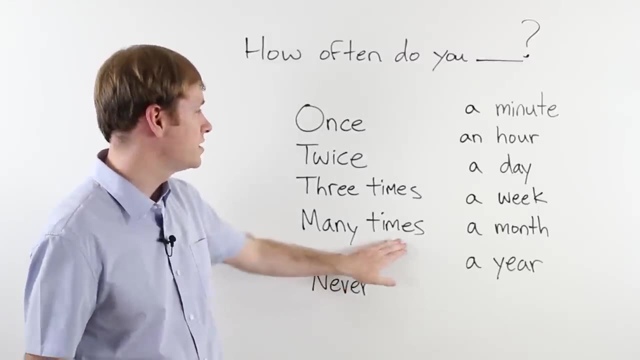 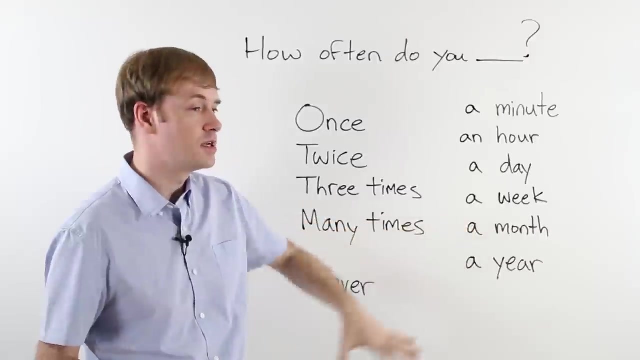 Four times, Many times, Okay, I eat a lot of food. I eat breakfast, lunch, dinner and some snacks. So many times a day, Alright, Okay. so that's, we're using a day a lot. Let's use one of these. 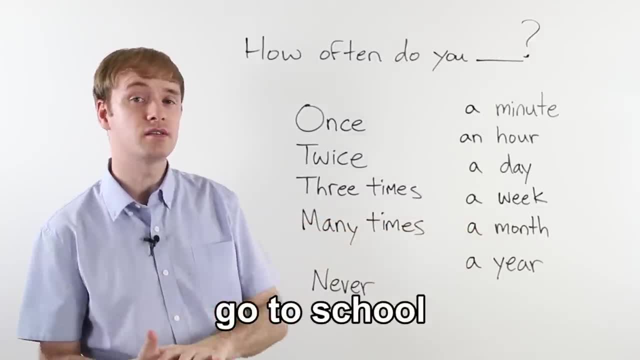 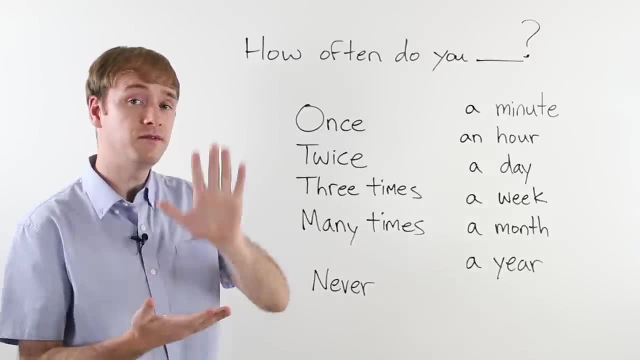 How often do you go to school? Okay, so, if I ask the question, how often do you go to school? Well, three times. If you go to school, maybe five times. Five times a week: Monday, Tuesday, Wednesday, Thursday, Friday. 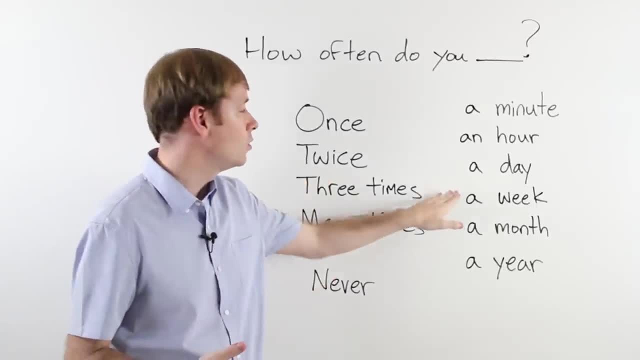 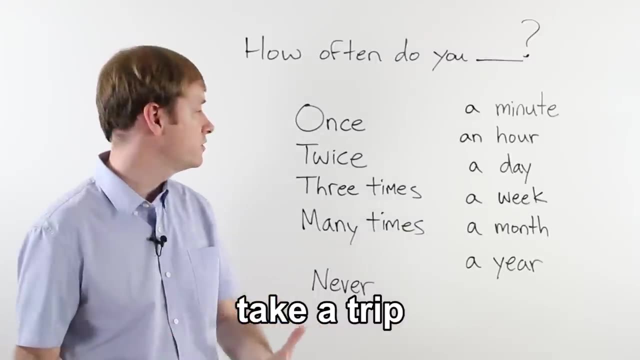 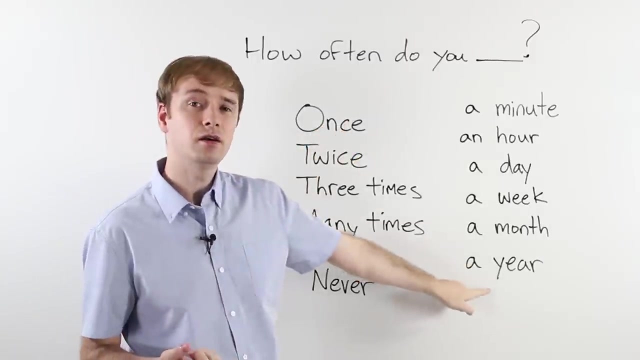 So you would say five times a week, okay. How often do you take a trip? Okay, how often do you take a trip? Well, maybe you would say once a year, Once a year, Maybe twice a year. Okay, 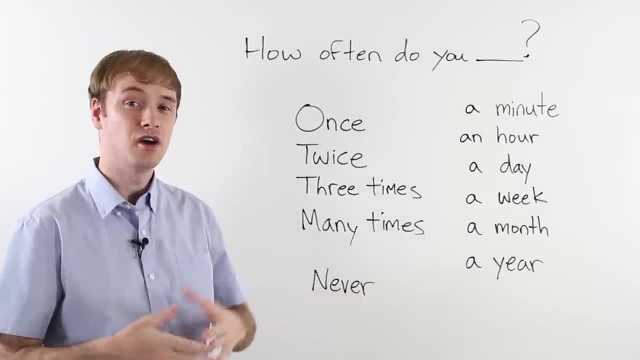 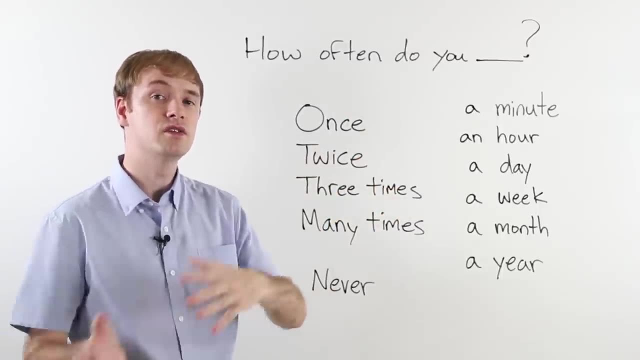 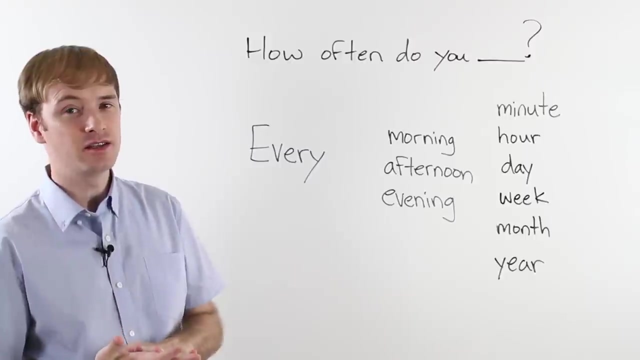 Maybe never? Okay, Never yet. never is also a choice. Alright, so this is how we use the definite adverbs of frequency. Let's move on to some more. Okay, we're going to look at the expression every. Every is very common, very easy to use, because you can say every morning, every afternoon, 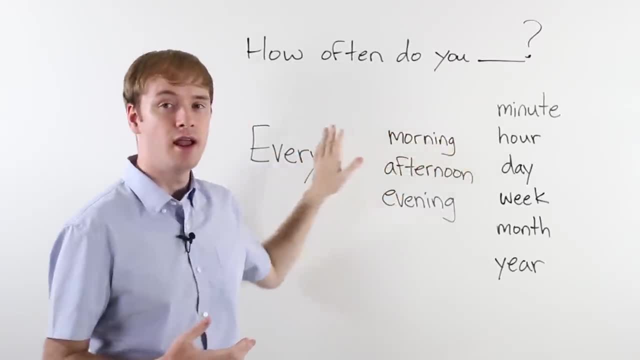 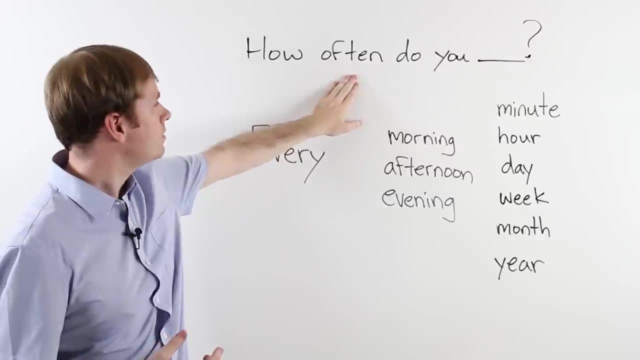 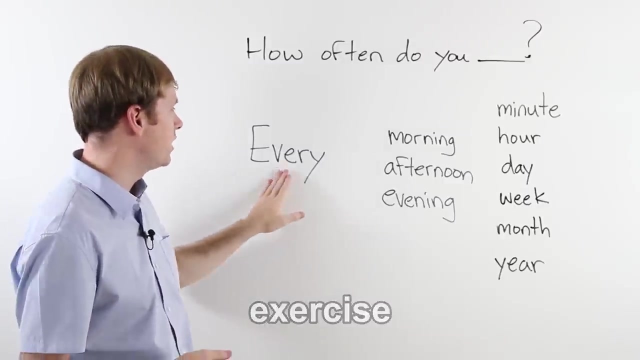 every evening, every minute, every hour, every day, every week, every month, every year. So Let's make a new question: How often do you exercise? How often do you exercise? Well, some of you maybe every morning or every evening, every day. alright, 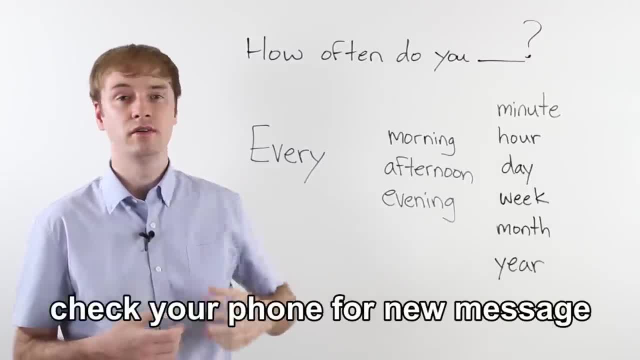 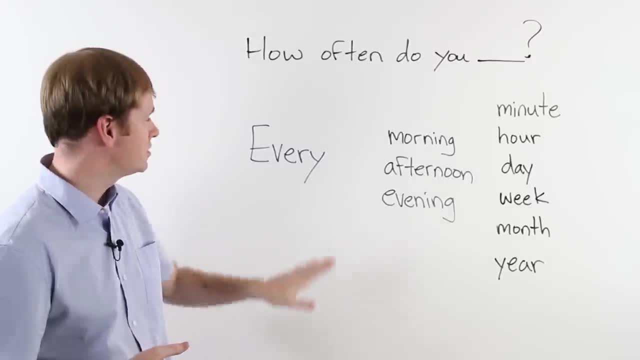 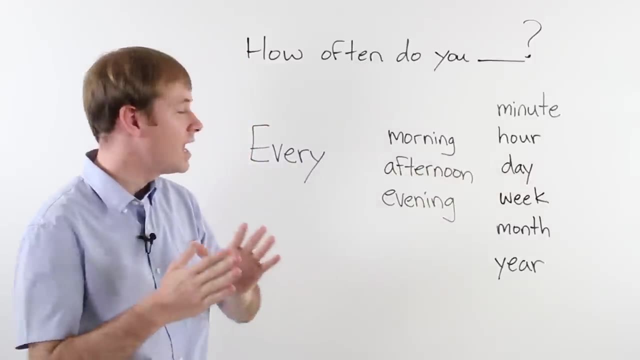 How often do you check your phone for new messages? Okay, so how often do you check your phone for new messages? Some of you might say every minute, Every minute I check my phone, Or every hour, Or every hour. How often do you visit your grandparents? 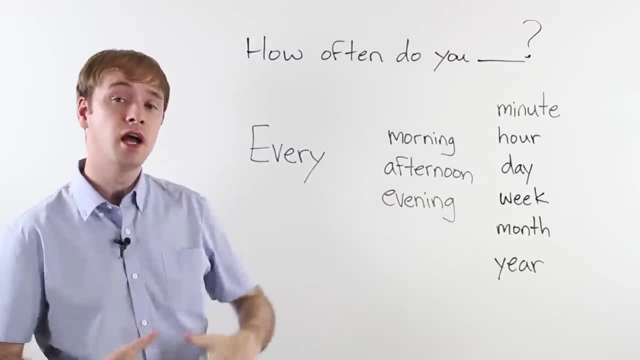 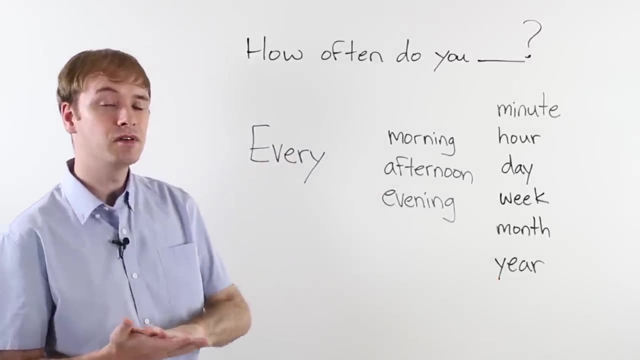 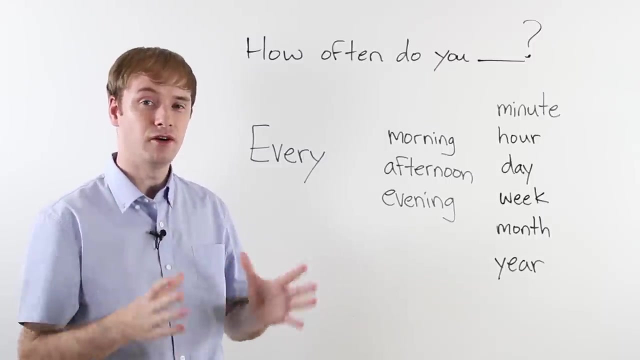 Okay, maybe your grandparents live very far. How often do you visit your grandparents? Well, every year, Okay, so that's similar to once a year Every year, Alright, so that's every Very easy to use, very common. 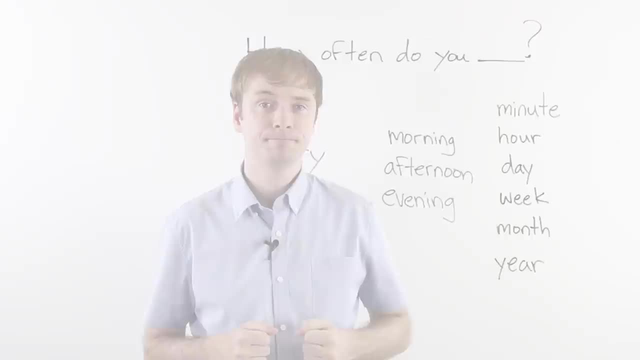 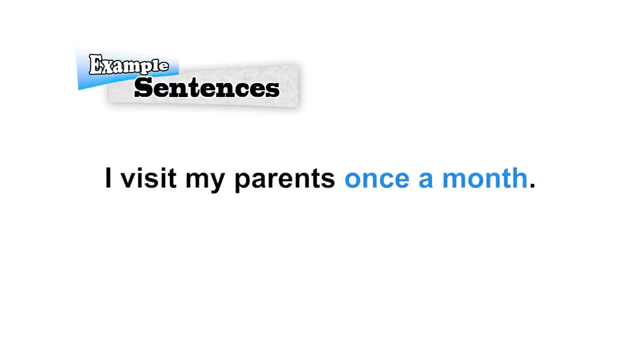 So let's look at some more examples right now. The first example: I visit my parents once a month. I visit my parents once a month. The next example: Five times a week I go jogging. Five times a week, I go jogging.